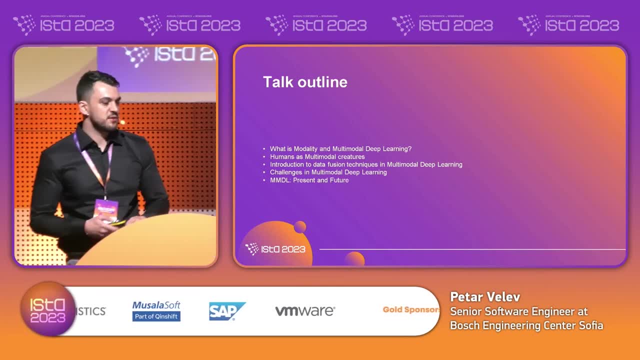 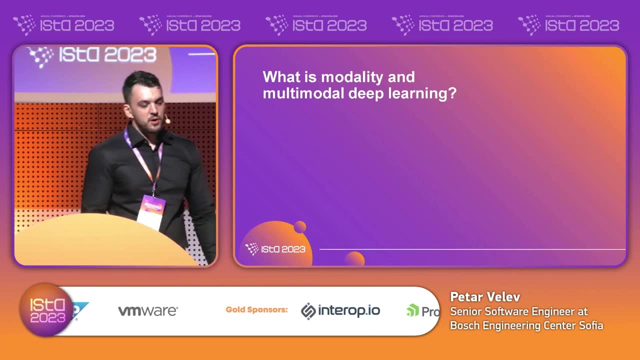 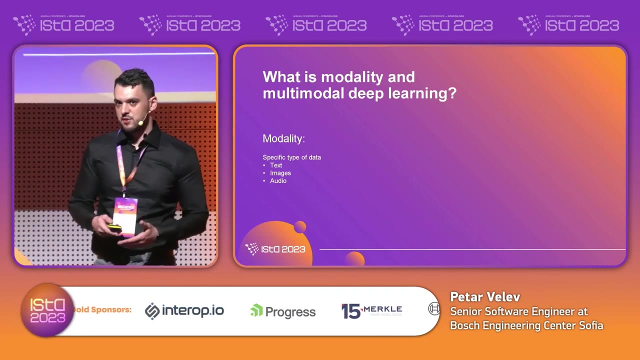 deep learning And at the end we'll see some real-world examples and what is in the future. So So, first thing first, what is modality? So, in the most simplest terms, modality refers to the different kind of data. For example, it can be visual data, like in images or video. 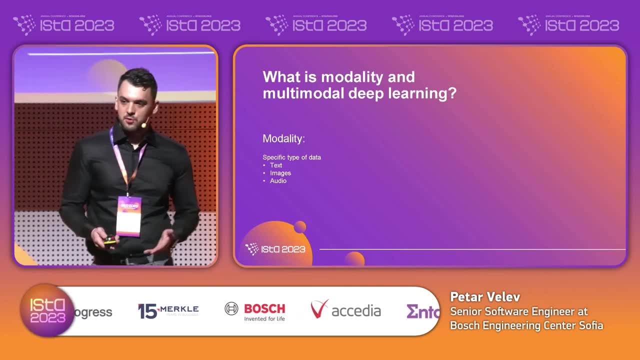 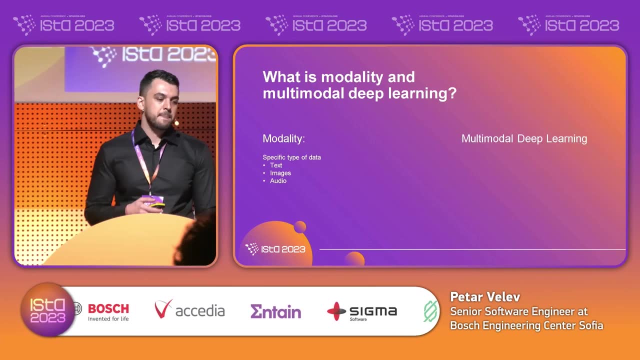 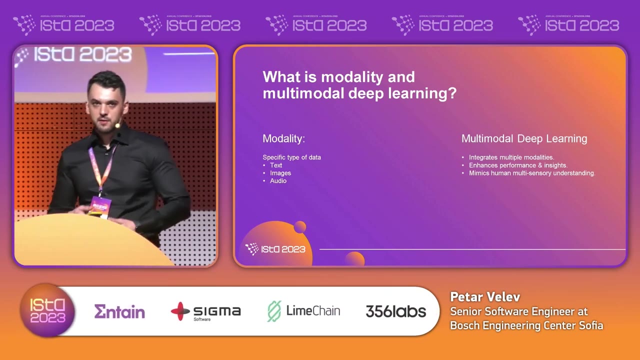 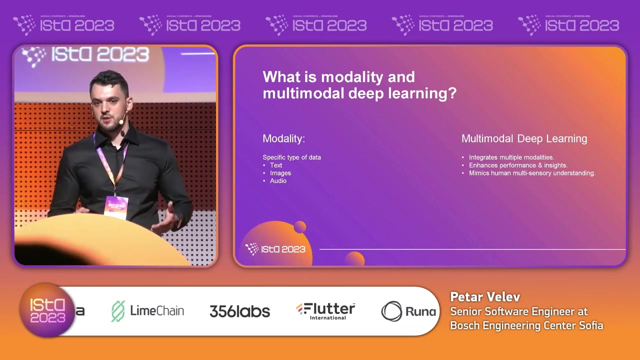 It can be audio data, like a song or a speech recording, Or it can be text, like you see in this slide, And multimodal deep learning is learning that involves multiple modalities. For example, this can be combining visual image information, for example, with text to generate a slightly different image, Or, for example, combining 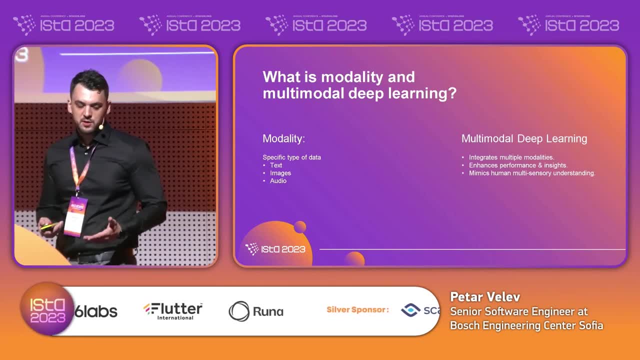 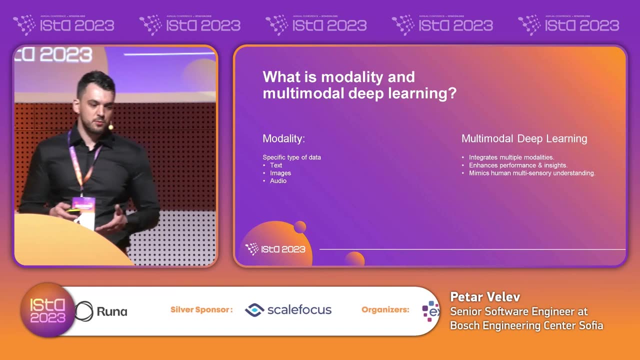 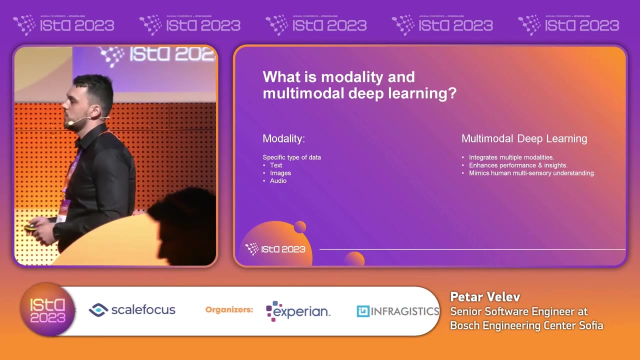 visual and audio information, like in audio-visual speech recognition, where one of the modality enhances the performance of the other, And it does quite well when it comes to when the environment is very noisy, for example. So So So, if you imagine you are a doctor and you have to diagnose a patient that has some sort 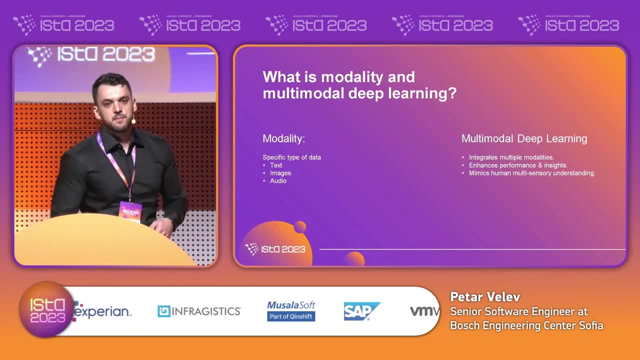 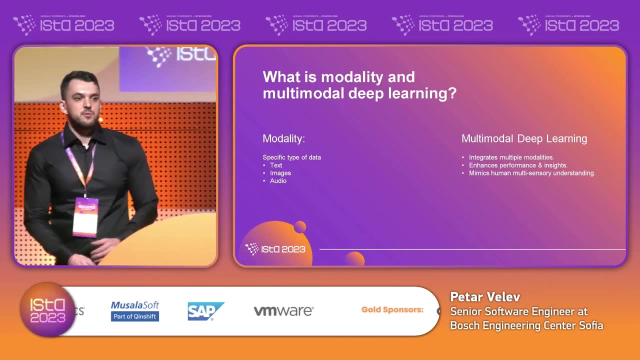 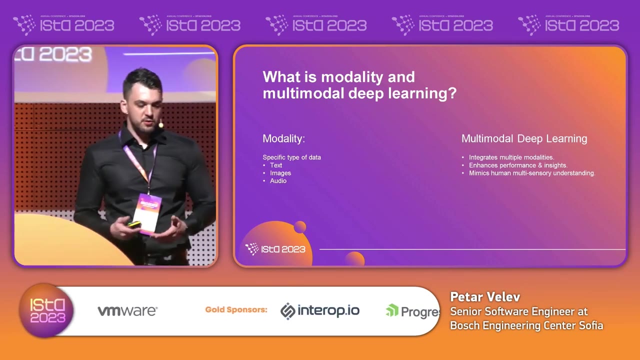 of lung problems. So which data will you use? Is it going to be the X-ray scan, the image of the X-ray scan, Or maybe it will be the audio information from your stethoscope that you heard, or some sort of audio recording of that? Or is it going to be the description? 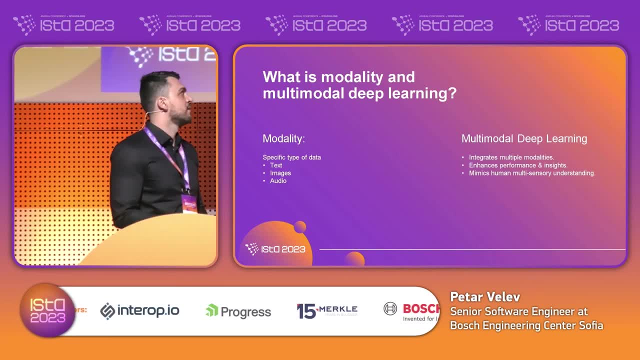 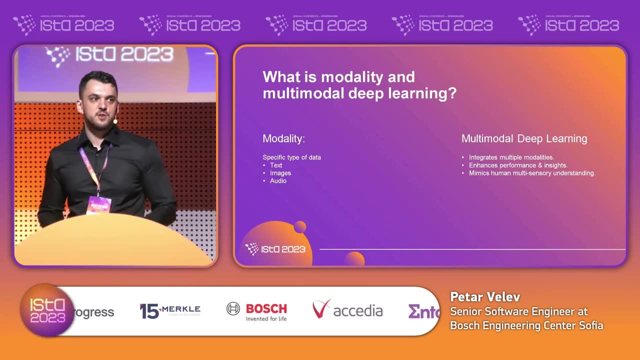 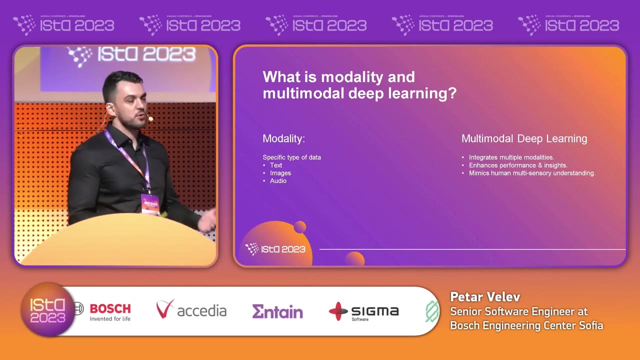 of the symptoms that the patient gave you. Well, hopefully, most doctors will agree that in order to give the best possible diagnosis, you have to use all of this information. So, in a sense, multimodal deep learning tries to mimic our human approaches to this kind of situations. And now I want to take a few. 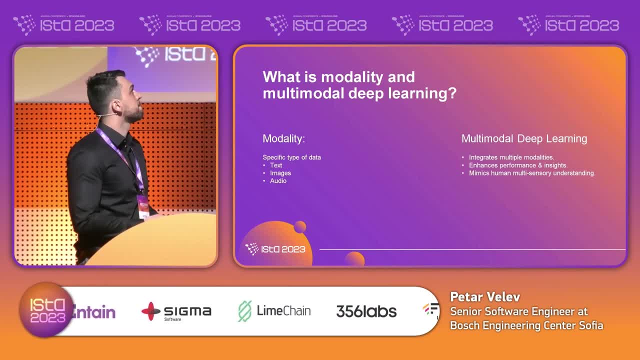 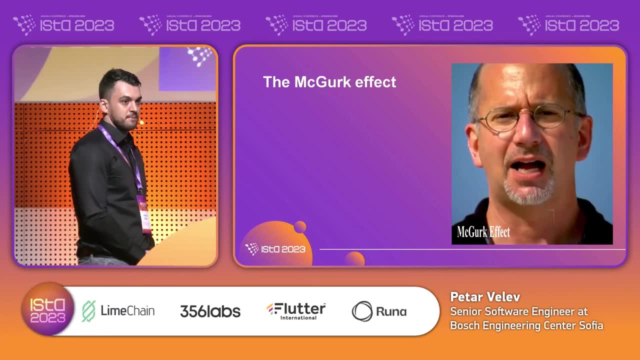 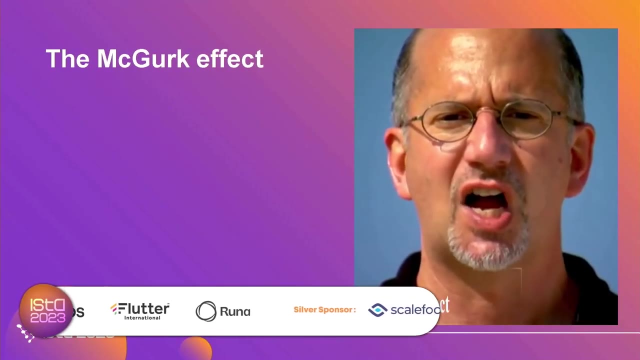 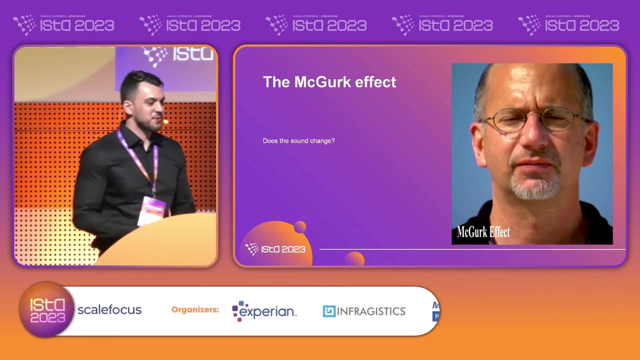 seconds to watch a video? So yeah. So how many of you heard different sound in the second clip? Yeah, So again, 50-50.. So those of you who paid attention to the screen probably heard different sounds in the. 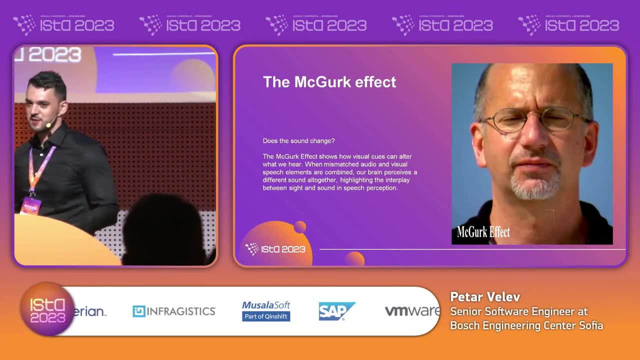 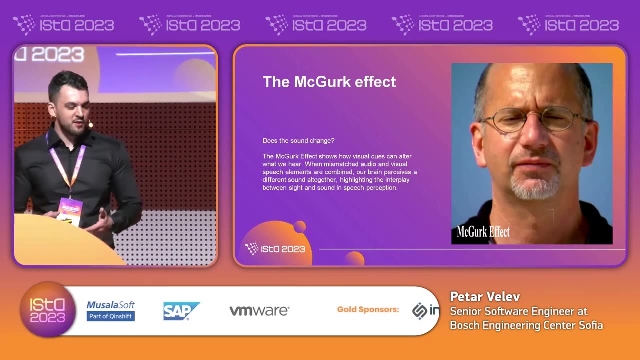 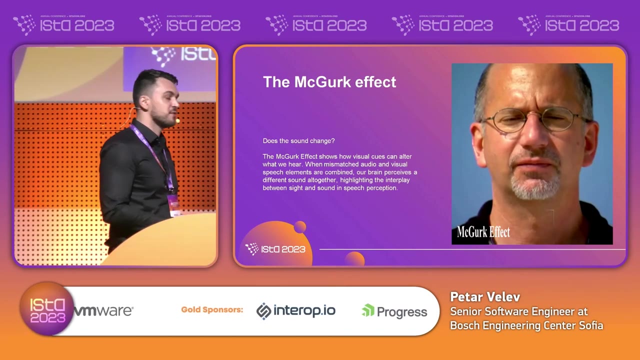 second clip, But for those of you who are just listening, probably it sounded just the same. This is called the McGurk effect And what it's showing is that our eyes can trick our ears, And it shows that we, as humans, we combine our sensory information to get this joint representation. 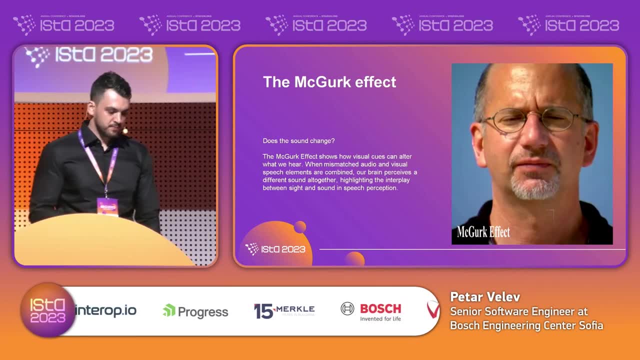 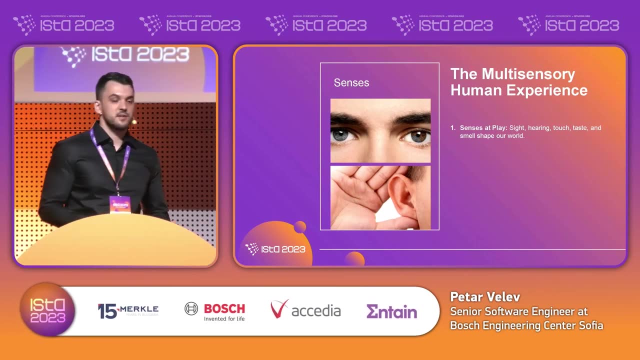 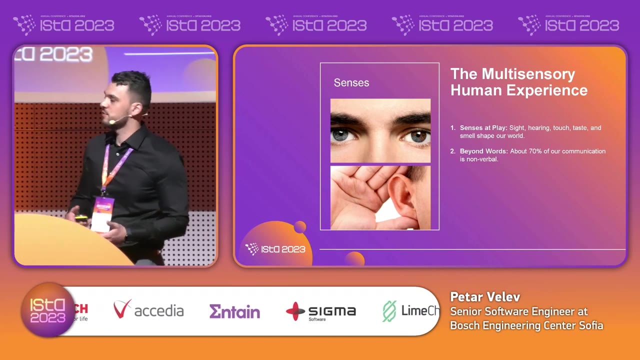 of the world And we combine. It's like sight, hearing, touch, taste and smell. And what is more interesting is that in our day-to-day communication, over 70% of it is actually nonverbal, which means that 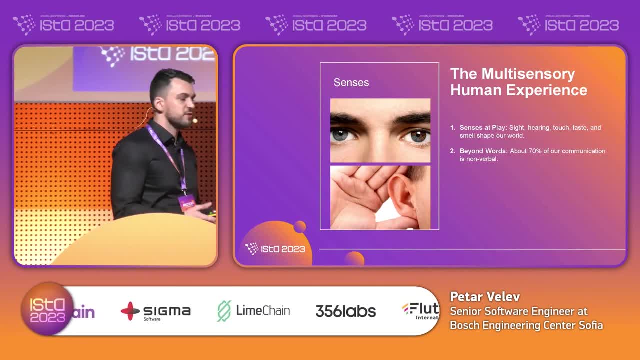 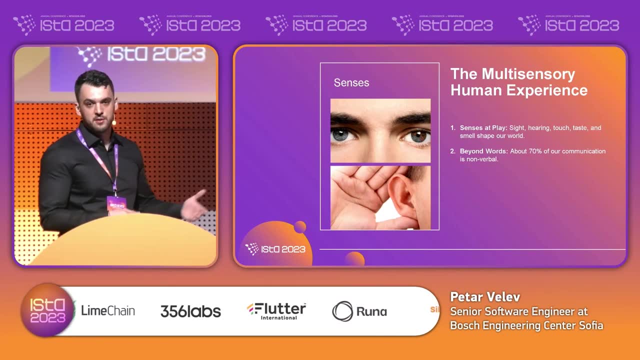 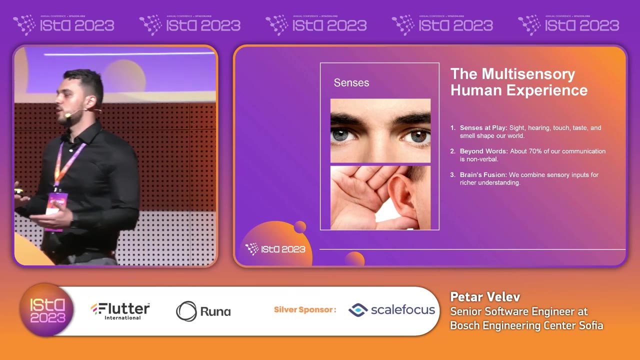 things like gestures, the tone of voice, eye movements and body positioning play a significant role in our communication, even more than the actual words that we are saying, And our brain is so good at fusing this information So we can have some sort of deductions and understand how a person is feeling or something. 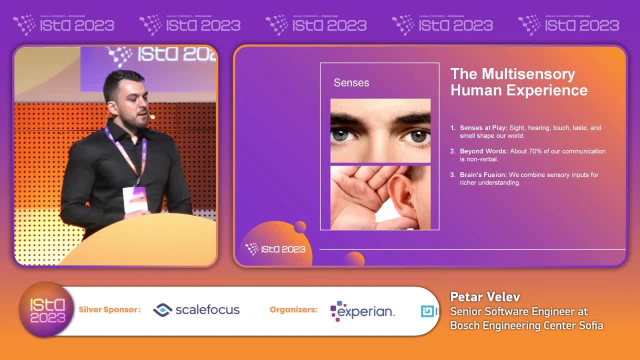 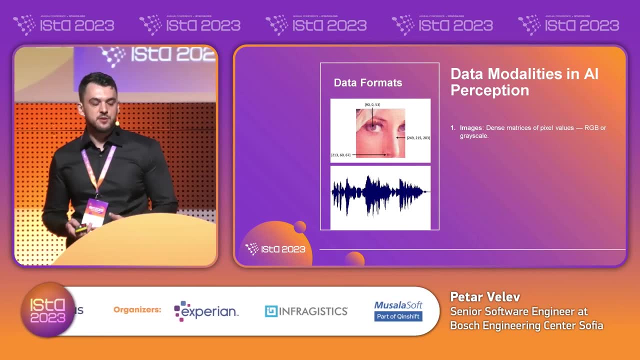 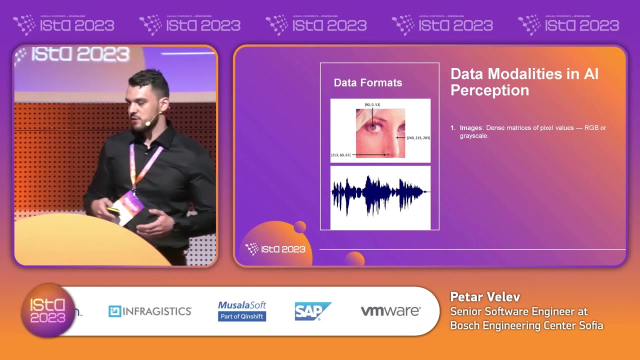 without he even saying this to us. So you know, AI, we have ways to represent this kind of information. For example, images and video, which is a sequence of images, is represented as dense matrices of pixel values, Like in the picture we see right here. 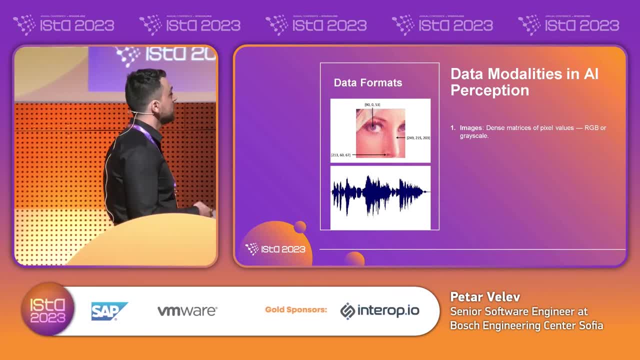 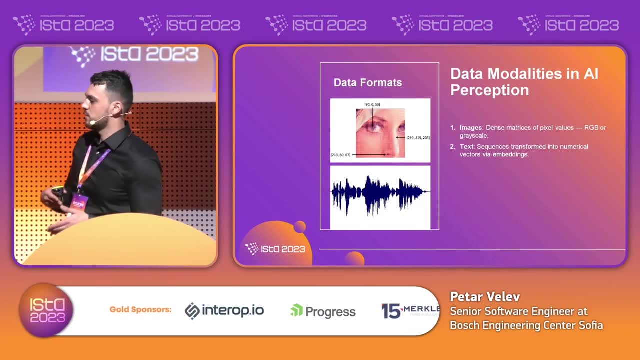 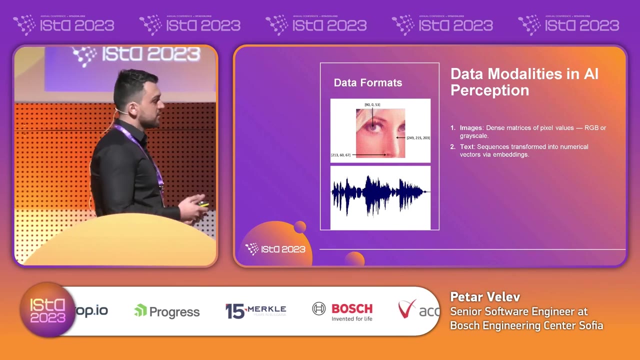 It's three values because it's RGB. If it's a gray scale, it will be a single value. Text, for example, is just a sequence of numbers that are actually digits in the computer memory And often in AI. we use embeddings to create this sort of numerical vectors to represent. 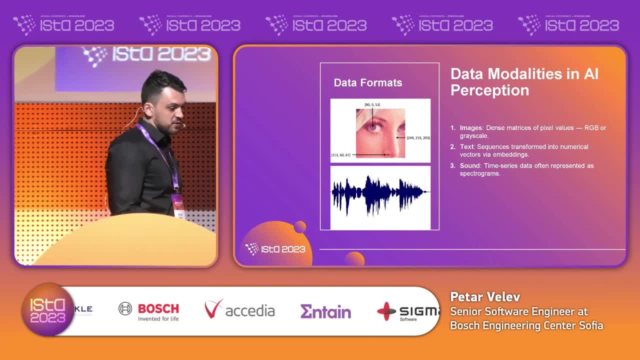 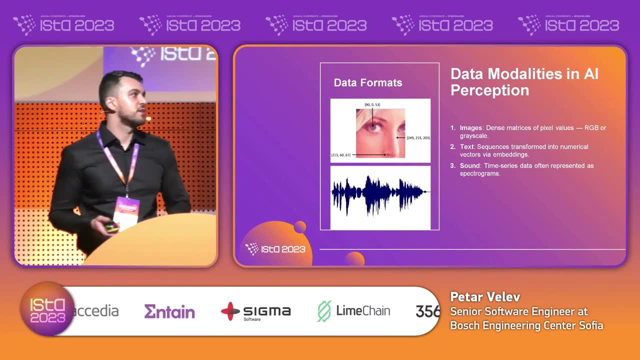 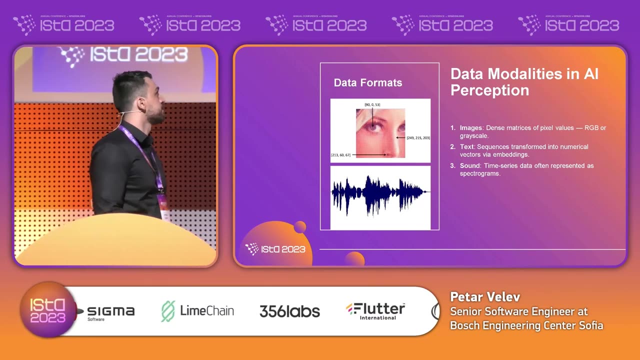 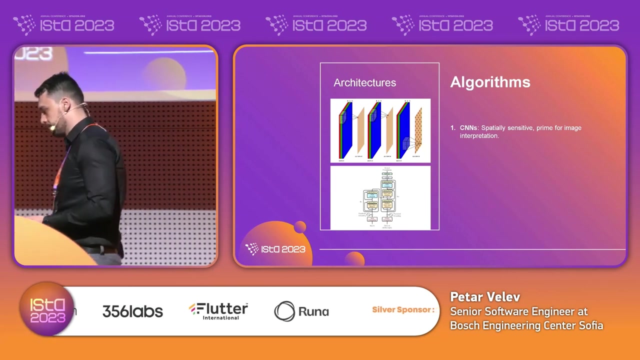 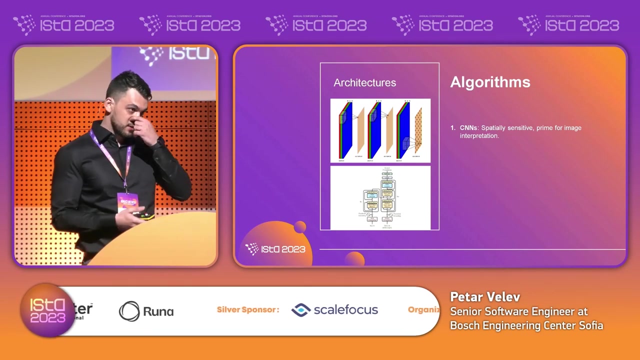 words And, for example, sound is a sequence of measurements And we often use. we convert it into spectral diagrams, spectrograms, using something like Fourier transformation, And we see great success with different algorithms. For example, convolutional neural networks are notoriously good for image classification. 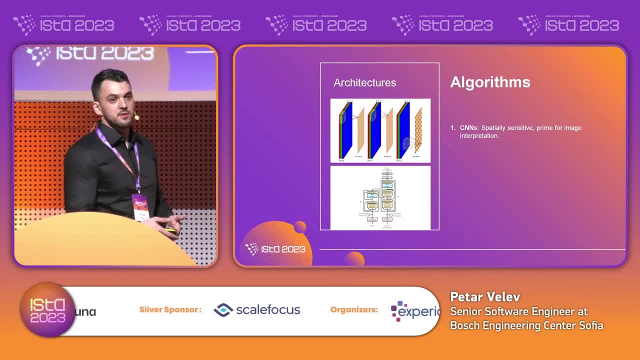 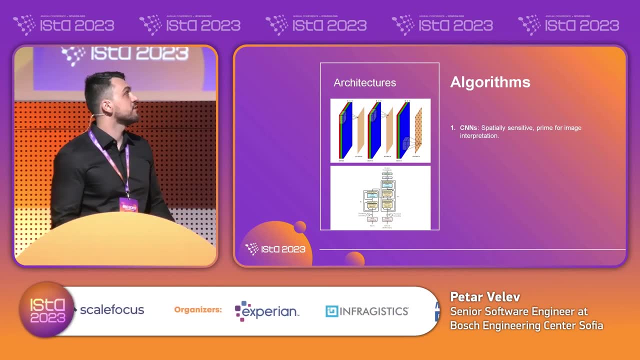 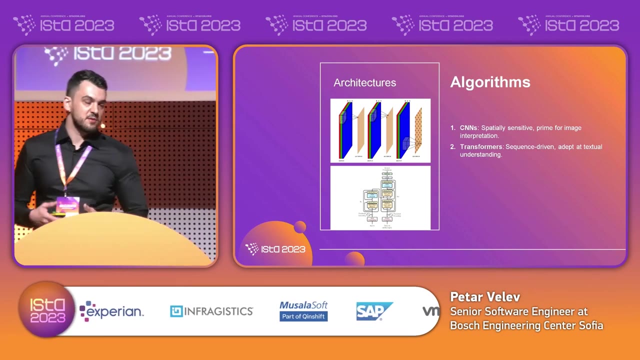 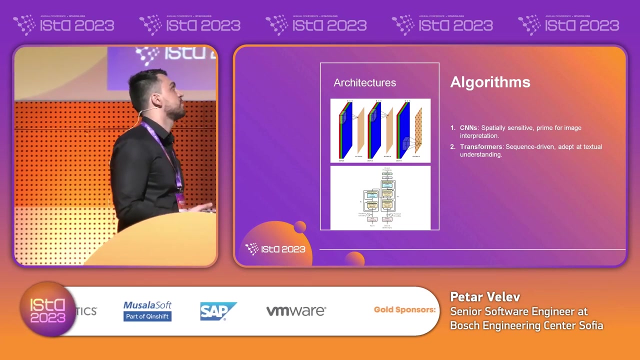 tasks and other image tasks Like object classification, Object detection, Object tracking, Even segmentation and image generation. Transformers are very good with language. We have seen things like chat, GPT and BERT, which are quite popular right now. Also, transformers have state of the art performances in other fields like visual and audio for 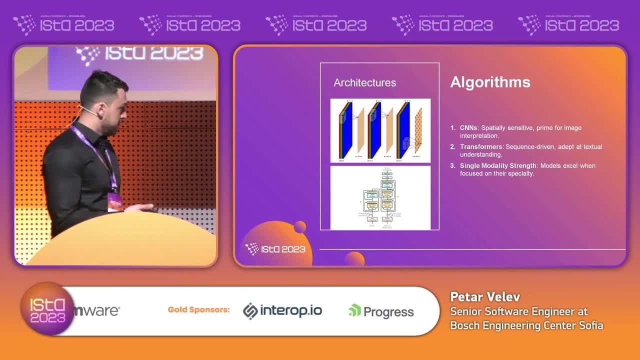 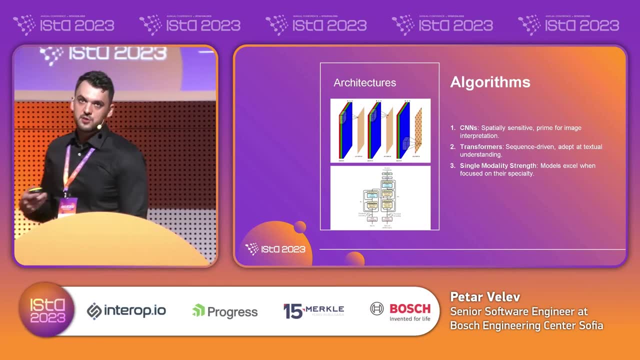 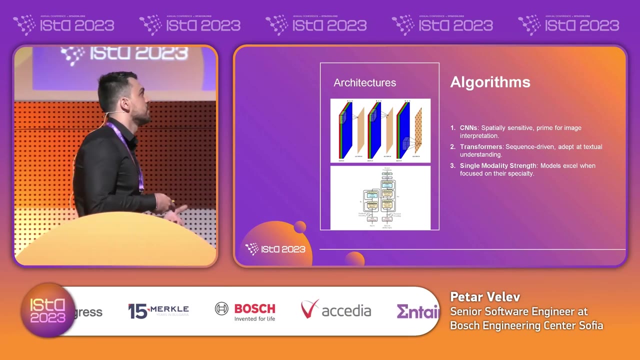 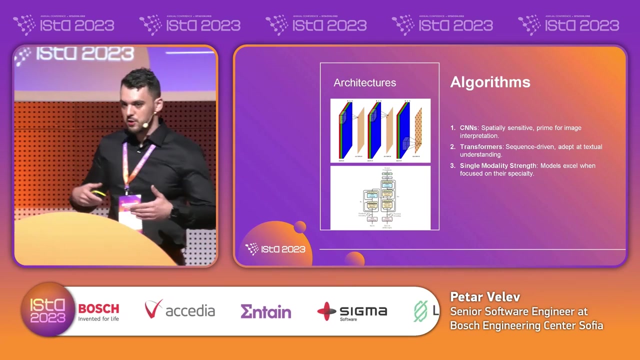 speech recognition, for example. Things like RNNs and their derivatives, like LSTMs and GRUs, are also being used for, for example, time series analysis or also speech recognition, And we see that all of these models are very good when working with single modality. 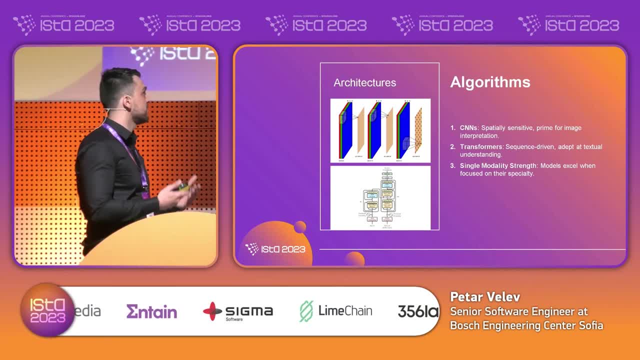 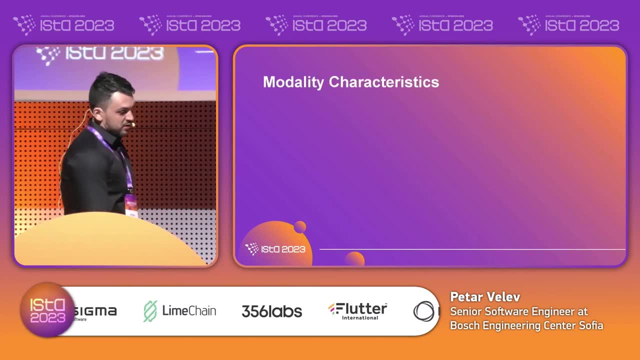 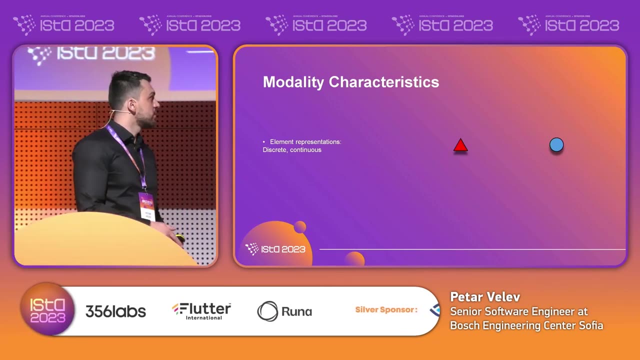 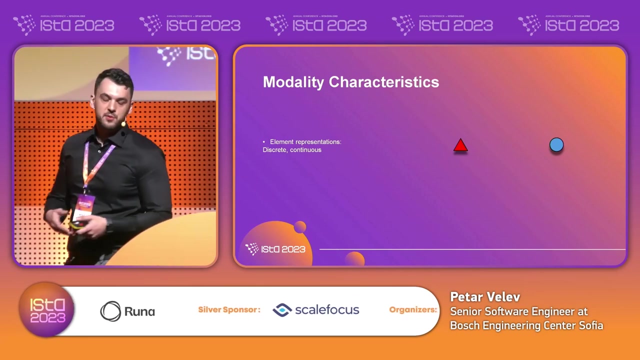 But they are good at capturing this essence of the modality. So let's see what are these characteristics of the modality. So modality characteristics: First one is element representation. For example, our elements can be either discrete, like for example in NLP, where each word 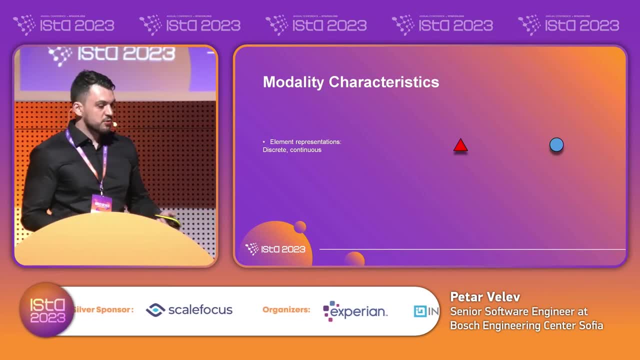 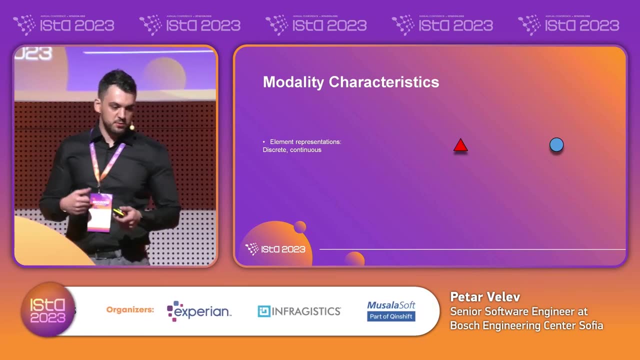 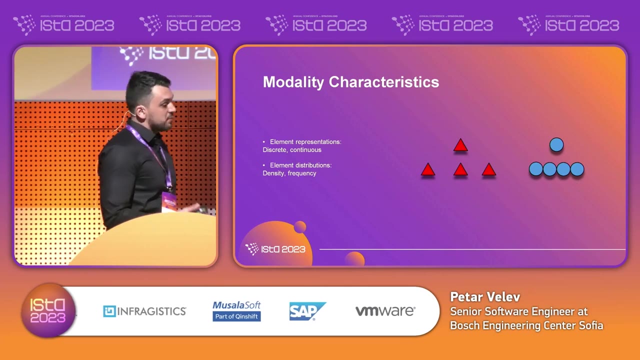 has its own distinct value, or each word or subword has its own distinct value, or continuous, like in the sound wavelength that we've seen, Where each value is somewhere between a range, Also element distribution. For example, is our data balanced or it's skewed in some sort? 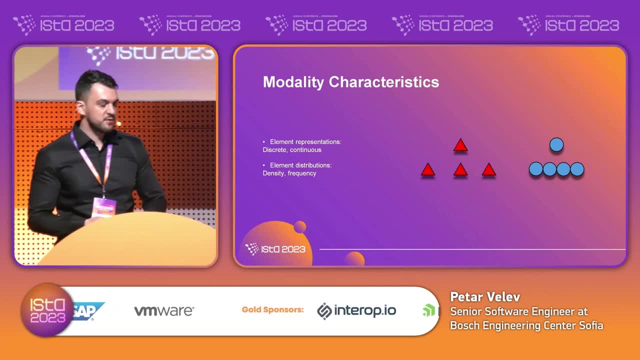 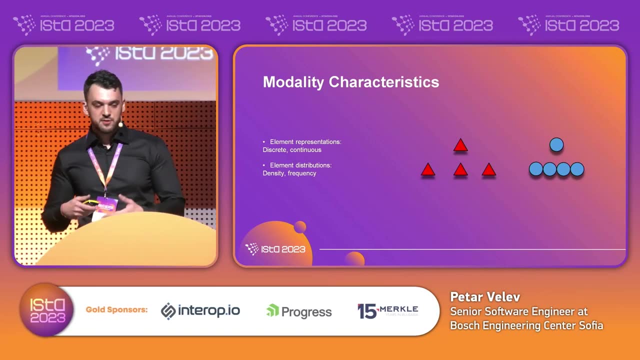 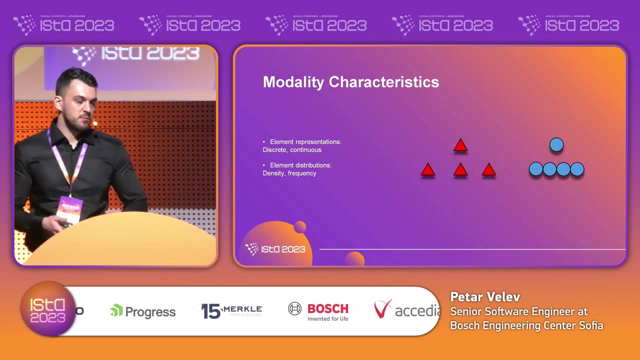 Do we have more of the same similar elements and less of some elements And frequency like, for example, do we see a lot of times the same elements, like in language, Some of the words are very often used And some are not used that often, like modality or multimodality. 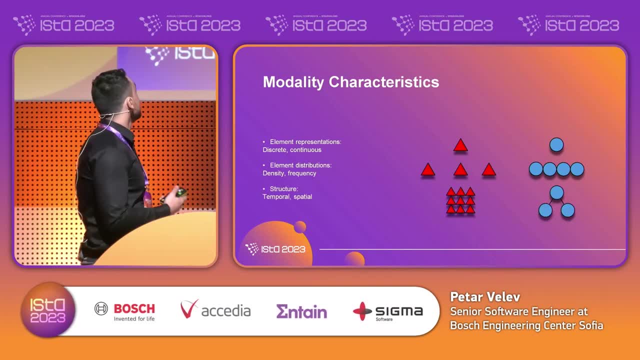 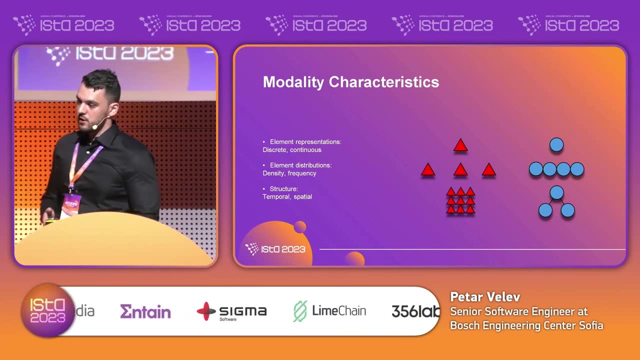 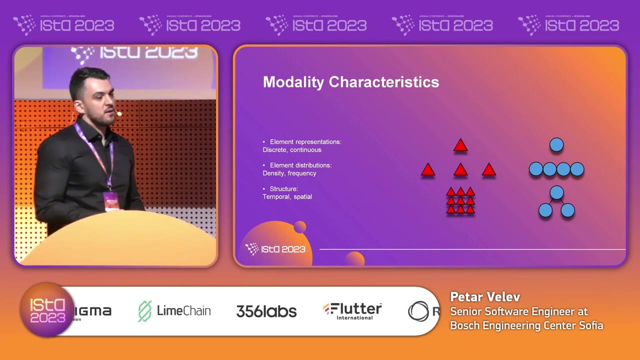 For example- it's a word that is rarely used, And the other thing is structure. For example, the structure can be temporal or spatial. Temporal, like in audio, where each distinct measurement has its order and the order holds information. Or spatial, like in images, where the pixels have their 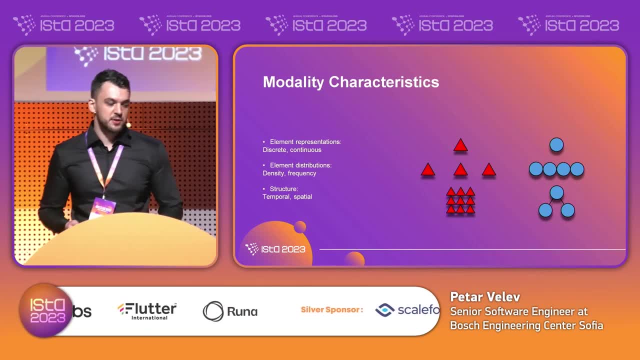 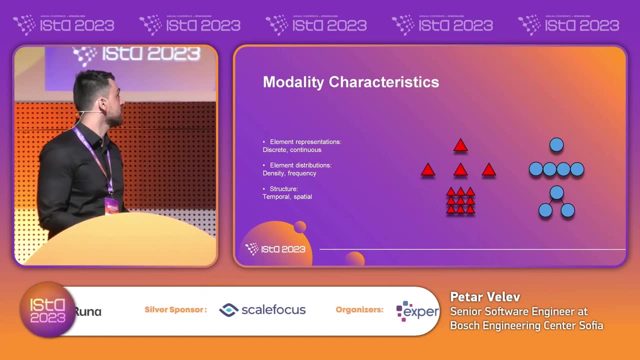 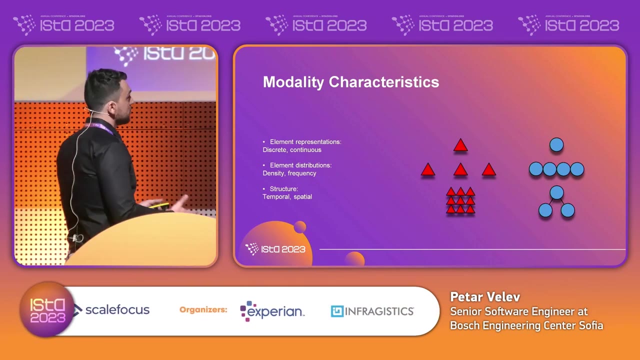 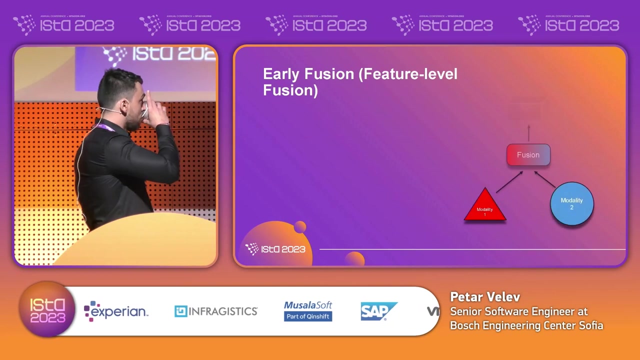 The pixel coordinates. The pixel coordinates are very meaningful for our algorithm. Hopefully now we understand that each modality has its own distinct characteristics And each modality has algorithms that work better with it. So now let's see how we can fuse this modalities to create a multimodal algorithm. 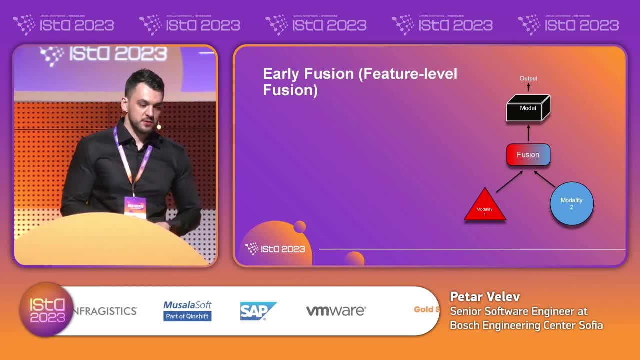 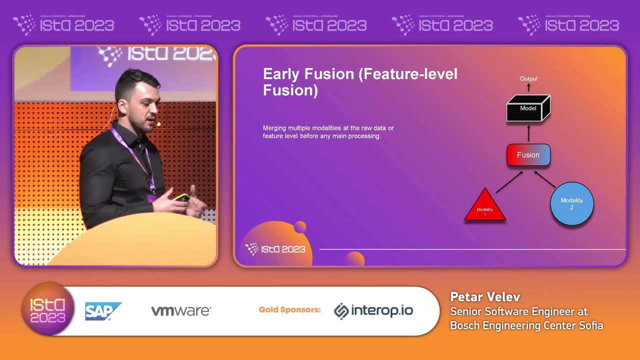 And the first. the proof that we can use is the early version. In early fusion, we combine the information at the very early stage, so we combine the features from both of the modalities before we pass them to our model, And this can be very simple. 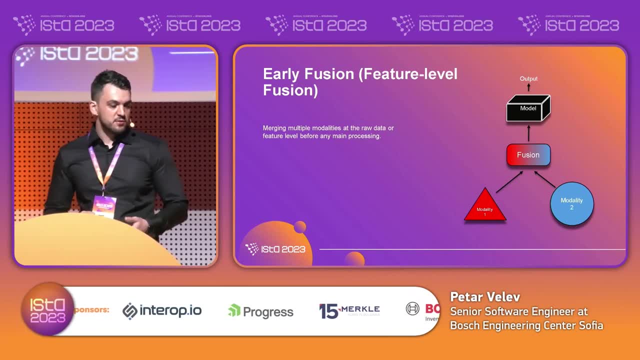 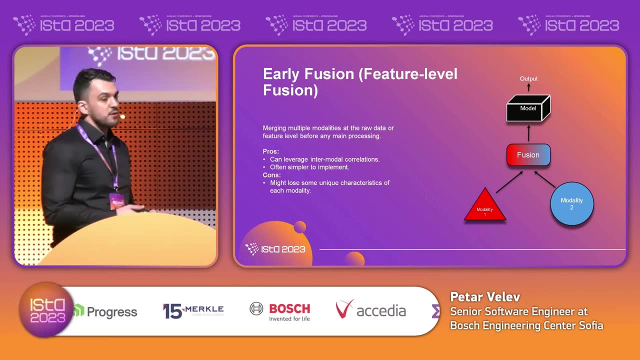 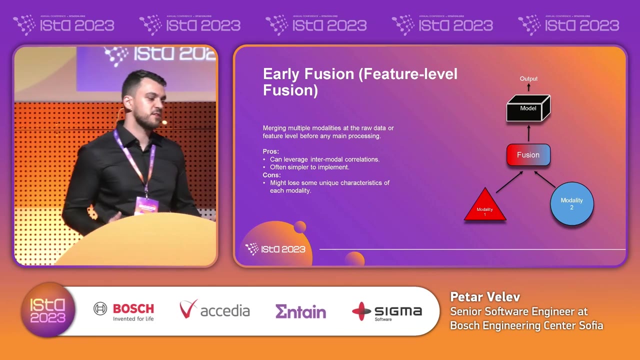 It can be something like concatenation, which is very simple, And the positive sides of this approach is that it's very easy to implement and it often can leverage these intermodality correlations very early on in the training, because we pass the data together. 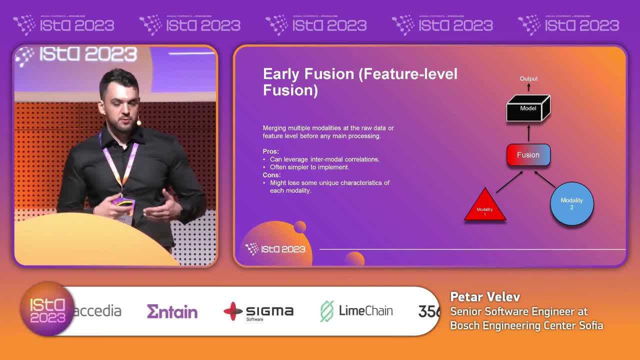 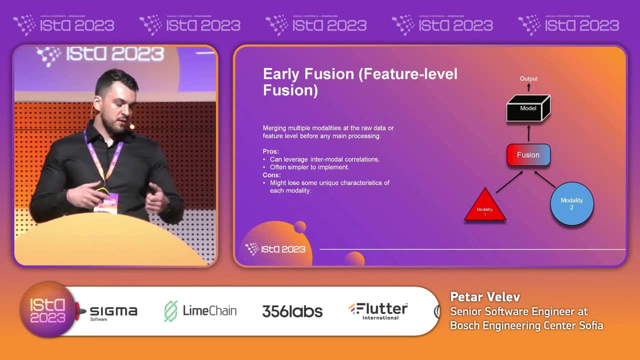 The negative side is that we might use some of the unique characteristics of each modality. For example, if we pass modalities that are temporal by nature and modalities that are spatial by nature. the algorithm is kind of getting confused with all of this information. 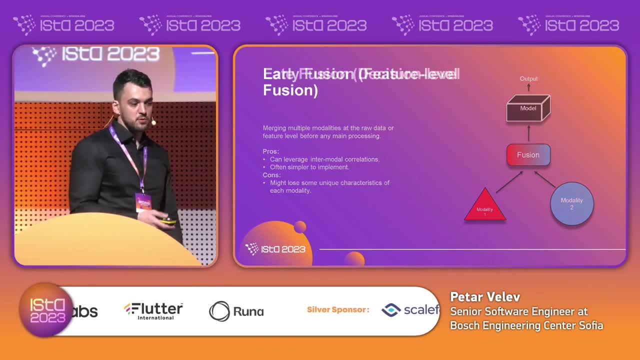 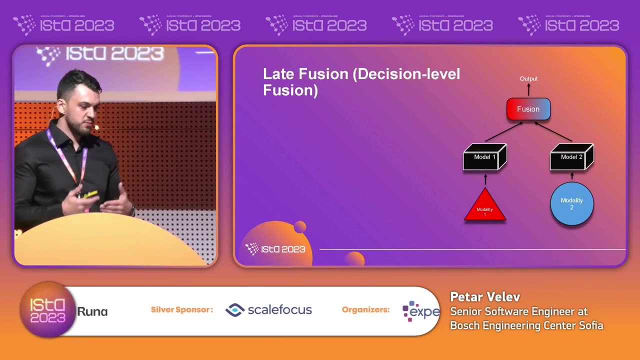 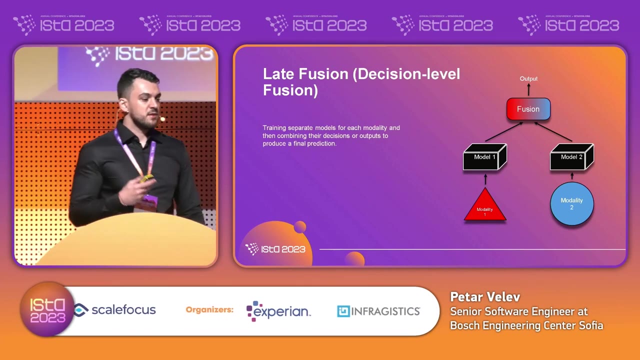 So if this is the case, we can use another approach, which is called late fusion. In late fusion we have we have separate models for each modality and the fusion step is after we actually do the modeling And the fusion strategy can be something like voting. 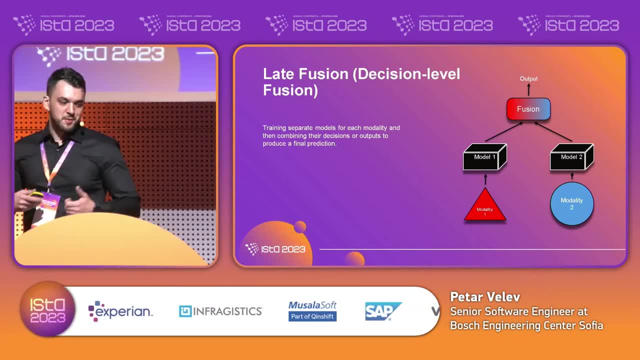 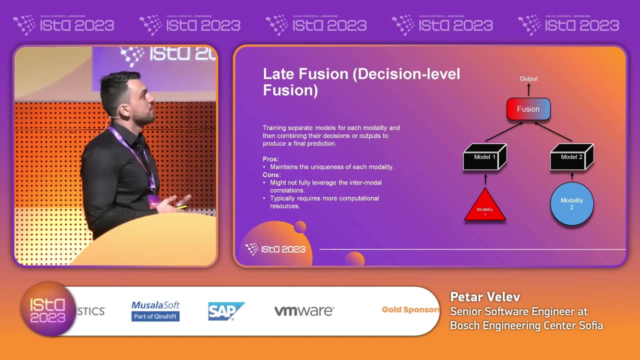 or some sort of a weighted sum or some different approach. The positive side of this is that it maintains the modality characteristic, since the model is dealt with the same kind of information, And the negative side is that it maintains the modality characteristic, since the model is dealt with, the same kind of information. 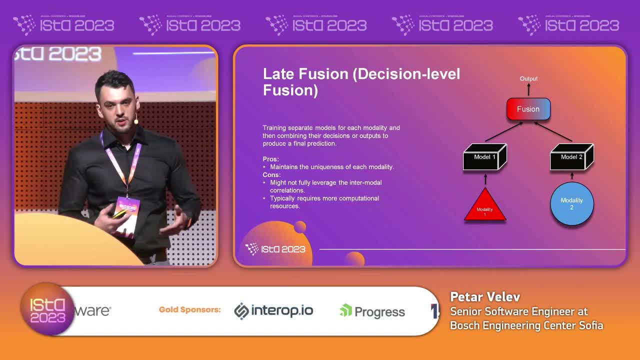 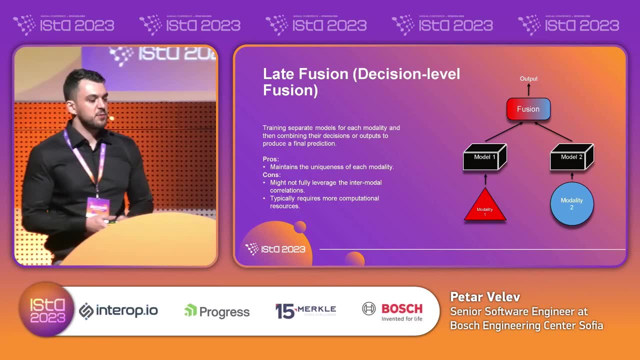 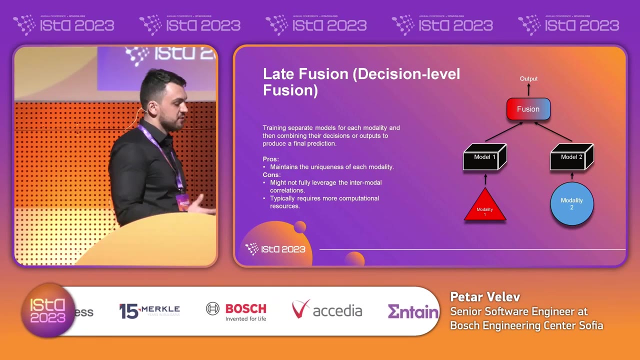 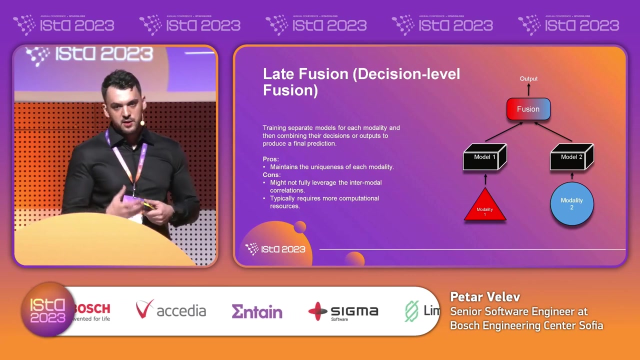 negative things is that it might not fully leverage the correlations between the different modalities, and also another negative side of this approach is that typically requires more computational power. for example, we do have to train on different stages. we have to train one model first and then the other model, and also, if we get some additional 5% better precision for 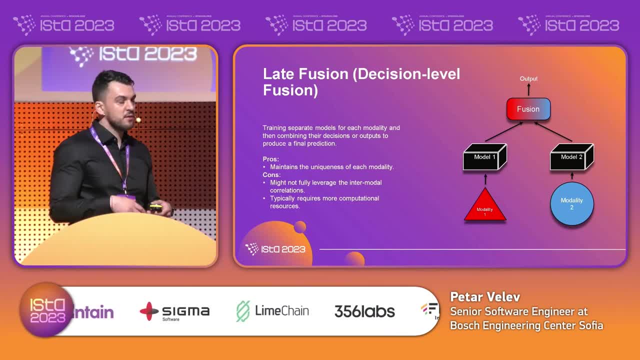 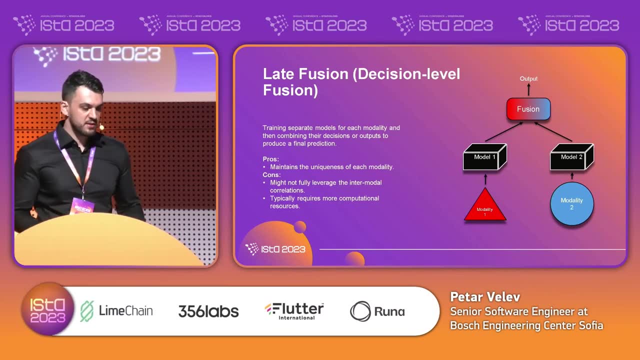 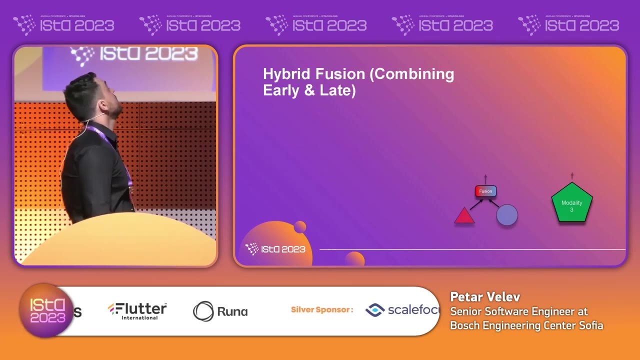 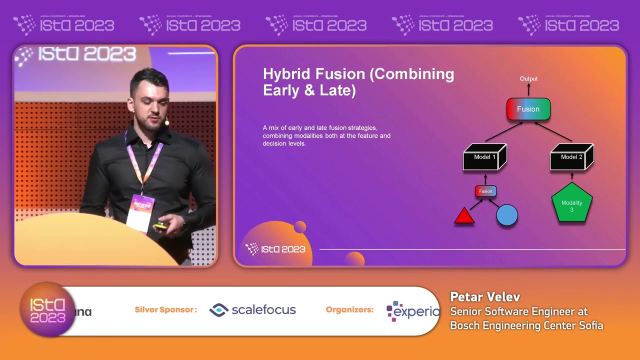 example. maybe for the most part we are doing redundant computations using the second model and just in those minor cases it it helps. another thing is hybrid fusion, for example. hybrid fusion aims to leverage the the positive side both from early and from late fusion, and it's very. 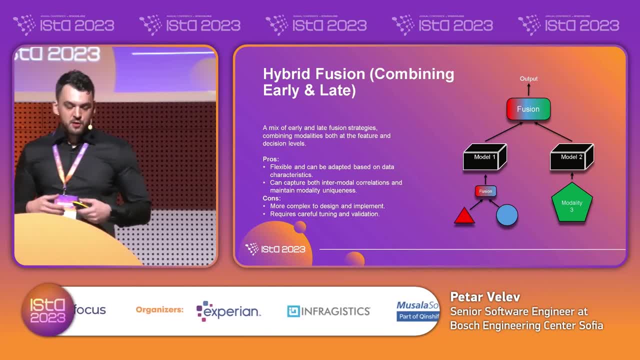 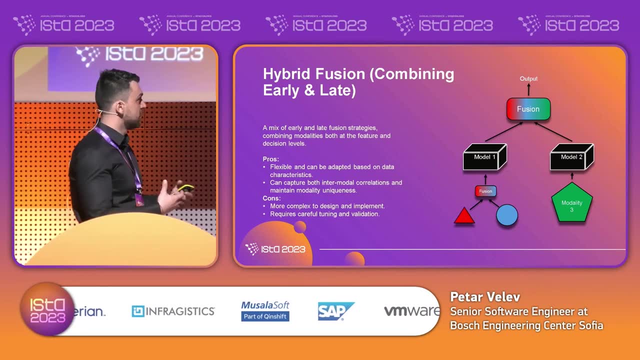 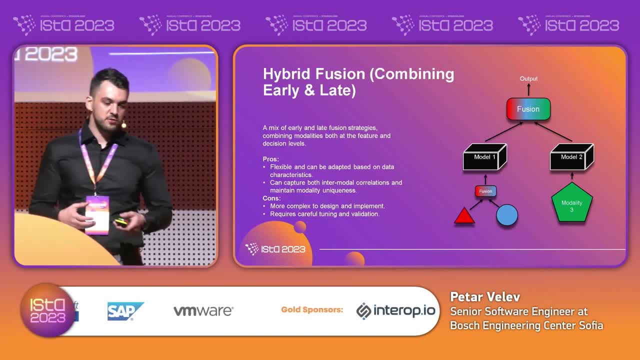 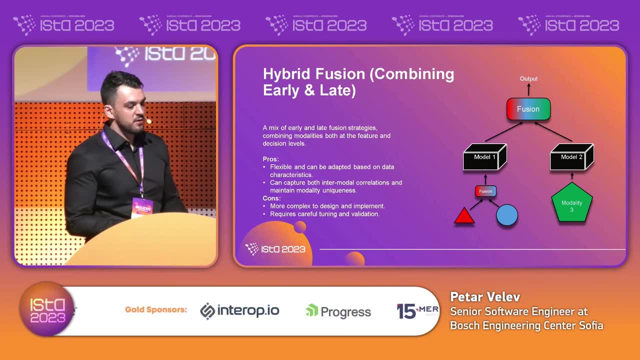 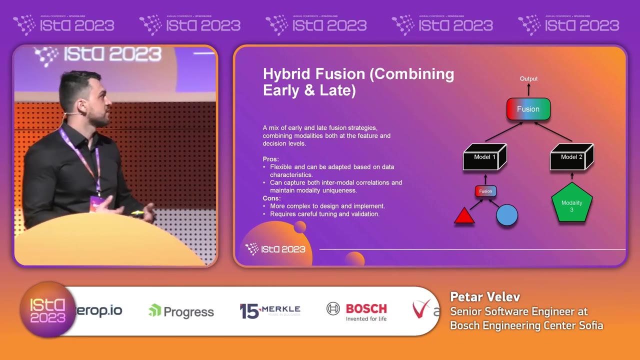 both of these models. we can use late fusion to actually get our output, and this is a normal use case, for example, in our day-to-day lives. the information that we see on the Internet, for example, has visual information, audio information and text information together. 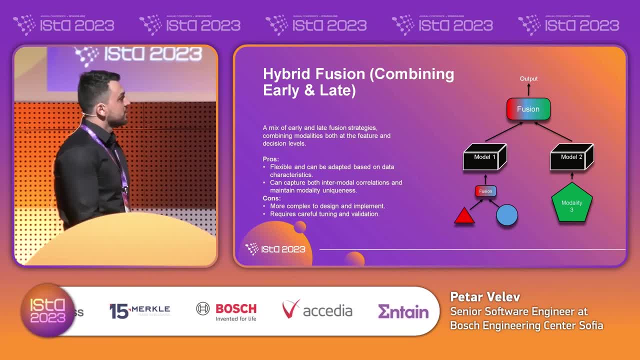 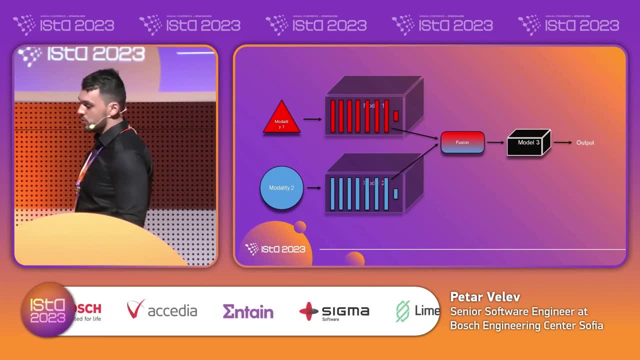 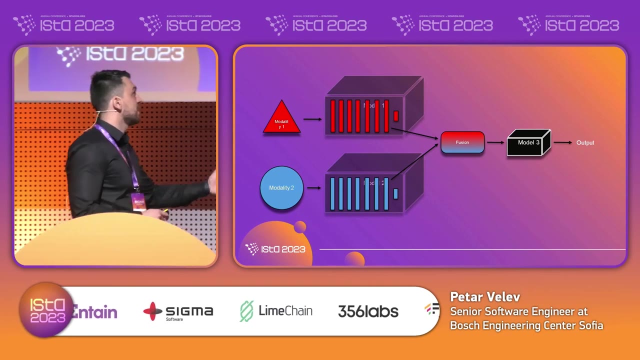 like in Facebook or Instagram, for example. This is a very possible use case. If we want to go deeper and get even more complex, we can use some intermediate approach and get not the last layer, like in Late Fusion, but get some intermediate representation. 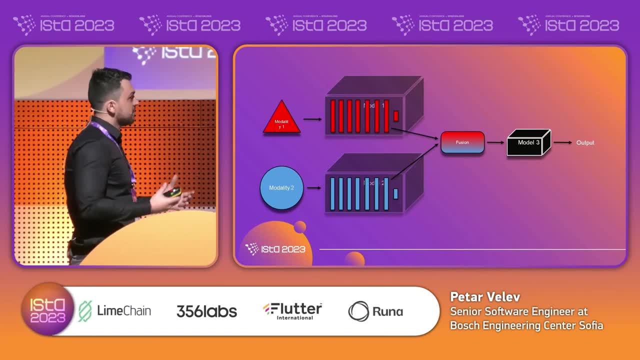 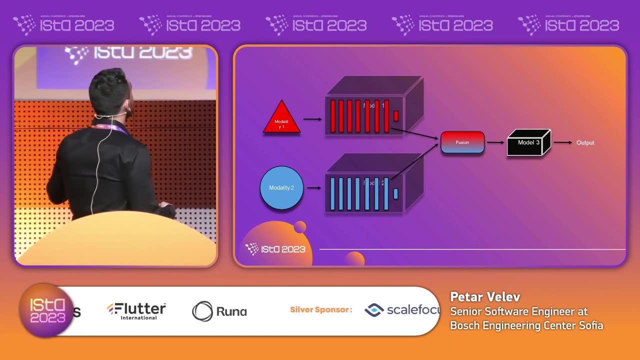 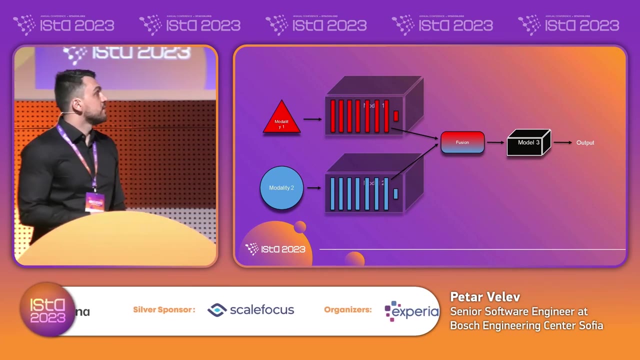 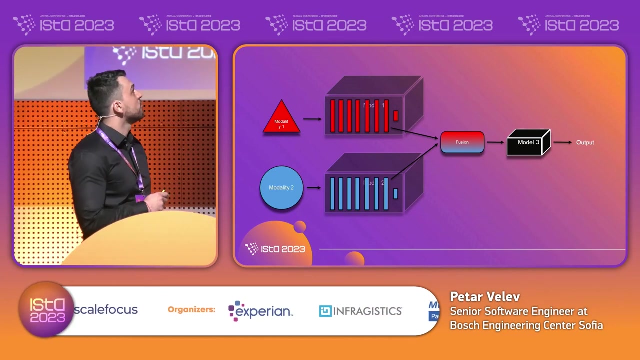 for example, from second to last layer. Then we fuse this specific information from the network, which is from intermediate representation, and then use another model to get our output. This is not the last thing. We can also use multiple layers from one of the models. 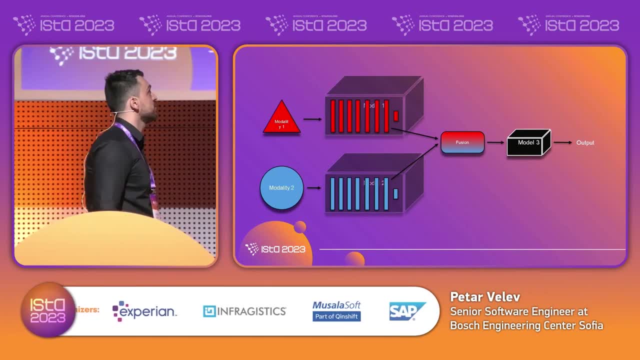 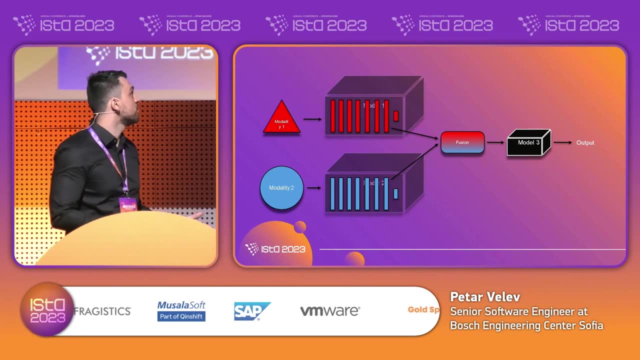 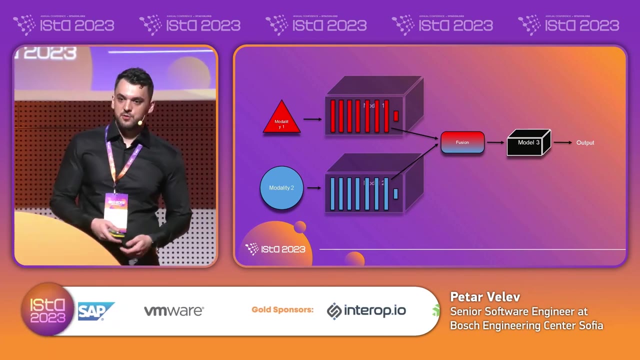 and multiple layers from the other model. This is also something that is used very commonly. Another thing, for example, here: if we really want to make it even more complex, the fusion mechanism, for example, can be something like attention, and this is called attention-based fusion. 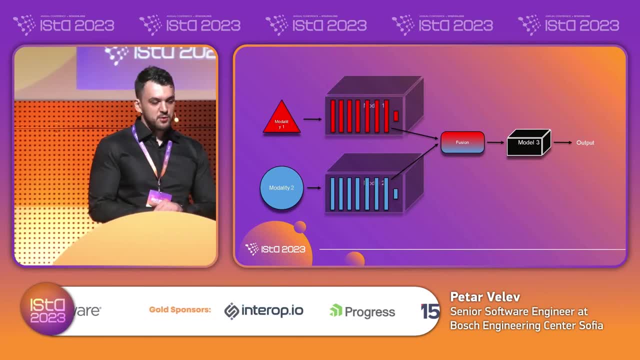 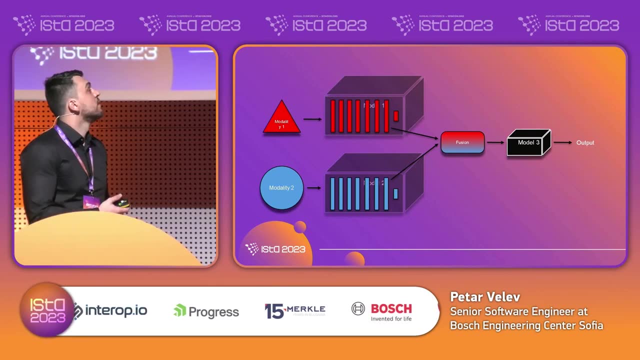 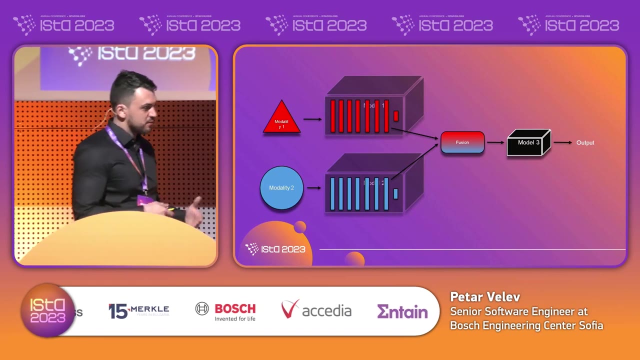 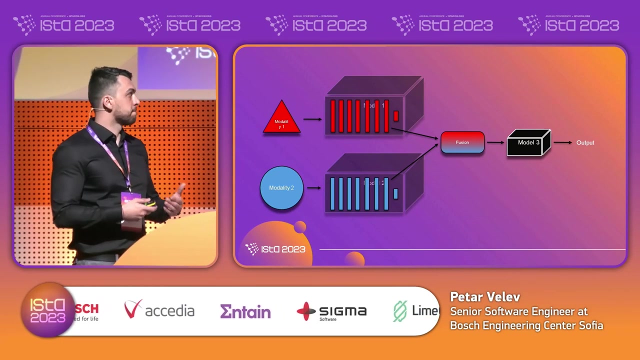 like in transformers. The idea here is that, with attention-based- for example, in the same example for audio-visual speech recognition, it's quite okay to use this, This approach, because, for example, where the environment is quiet and the audio information is very good. 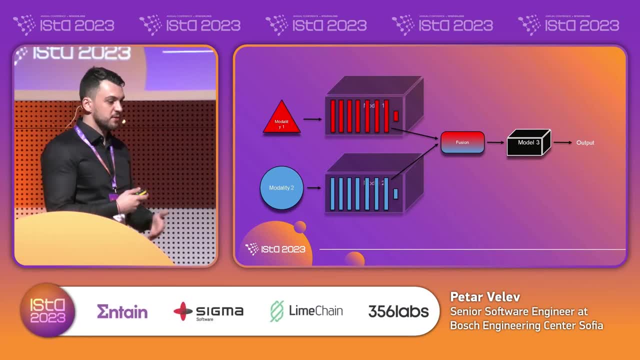 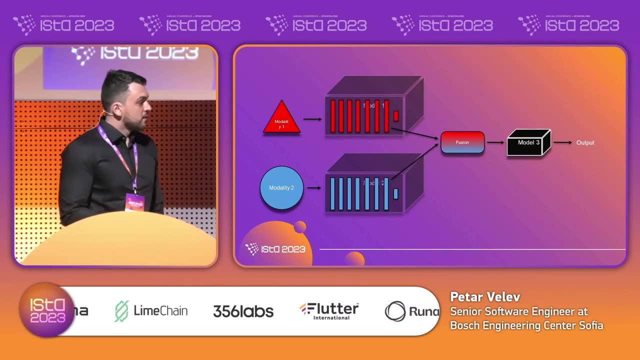 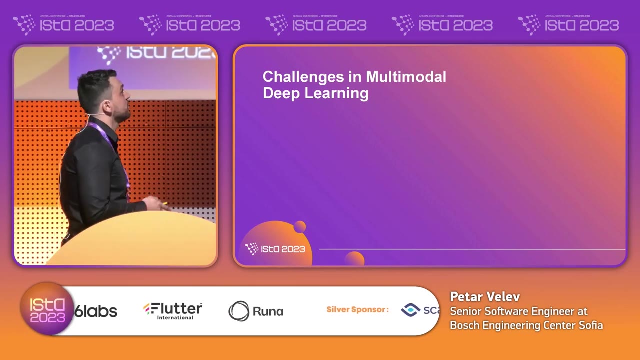 we can use the audio information, but when there is a noise in the environment, the attention mechanism can decide to use the visual information more than the audio information. What are the challenges in multimodal deep learning? Well, first, it's complexity. 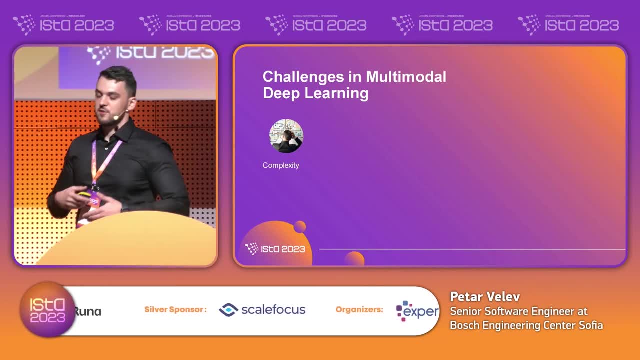 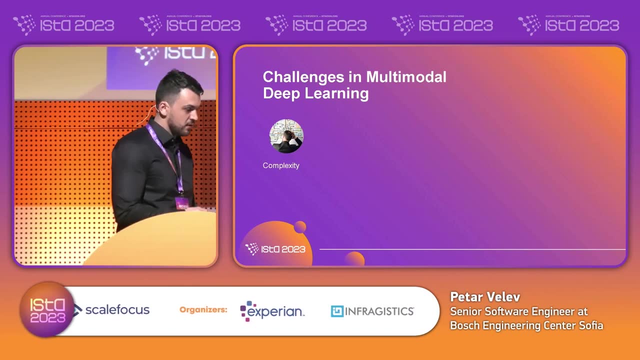 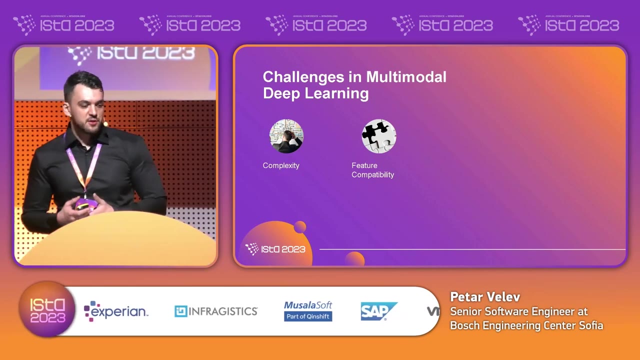 It's usually more complex to design such systems. They are quite difficult, They require more power, They are quite difficult to evaluate. The other one, for example, is feature compatibility. It's very difficult to combine modalities with different characteristics, For example, if you want to have a meaningful fusion. 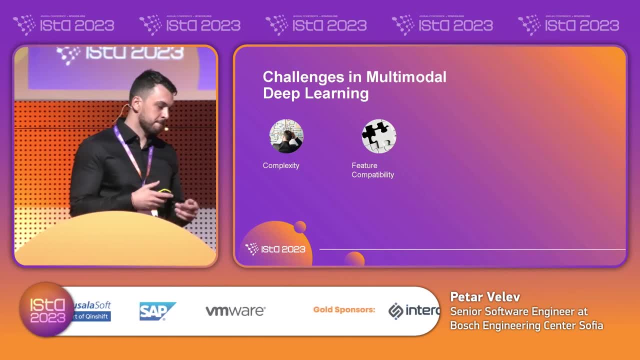 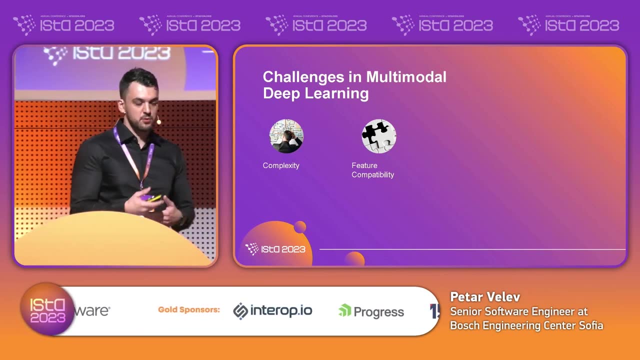 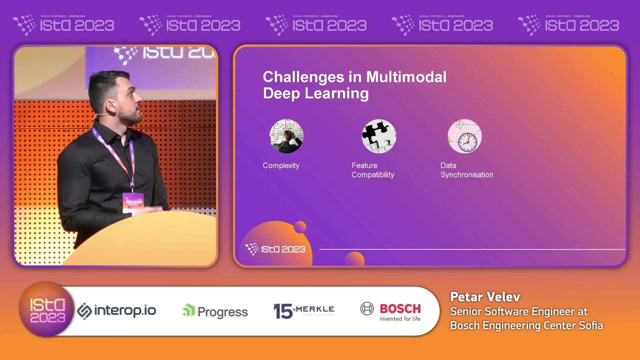 between modalities who has, for example, one is discrete and the other one is spatial and the other one is continuous. for example, we have to do a lot of transformations and normalizations to achieve meaningful fusion Data synchronization with the same example. 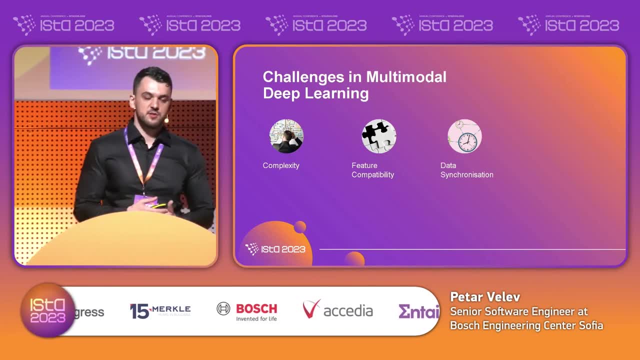 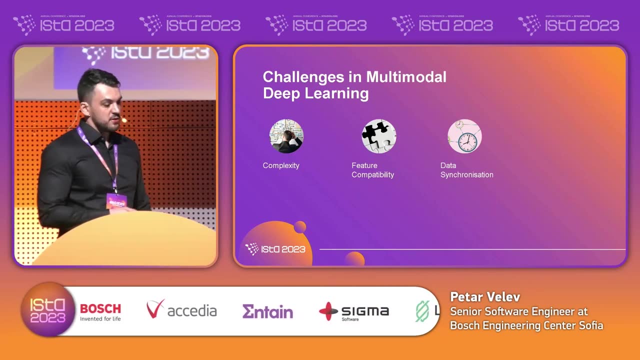 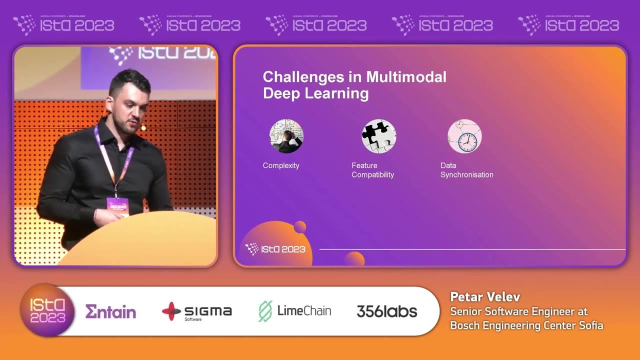 with audio-visual speech recognition, for example, when we pass our individual point of measurement, our individual unit that we pass to the network, it's very crucial to be very well synchronized, or either it will make the network teach on wrong data Computational power with bigger models. 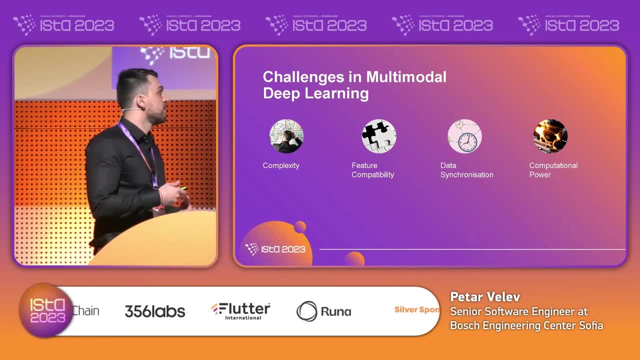 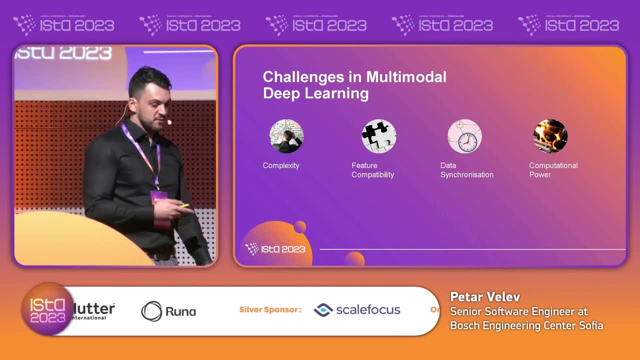 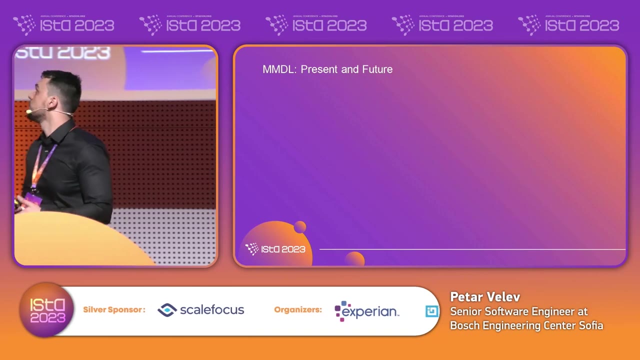 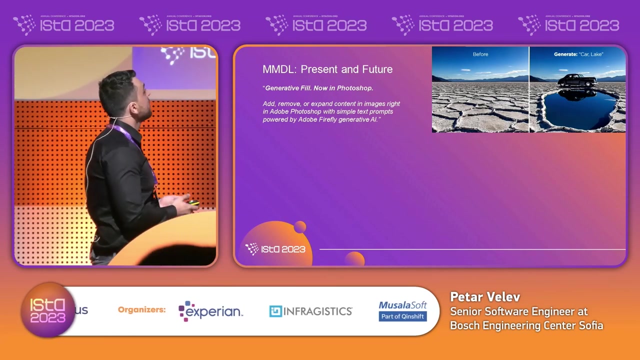 it's normal to require more computational power. We usually need different steps of training, like multiple training iterations, to achieve our results. Yeah, Hopefully this is a nice introduction to this field, and now we can see some real-world examples. The first one is one that I find fascinating. 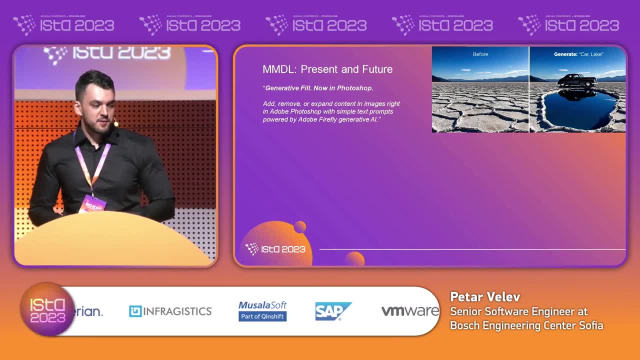 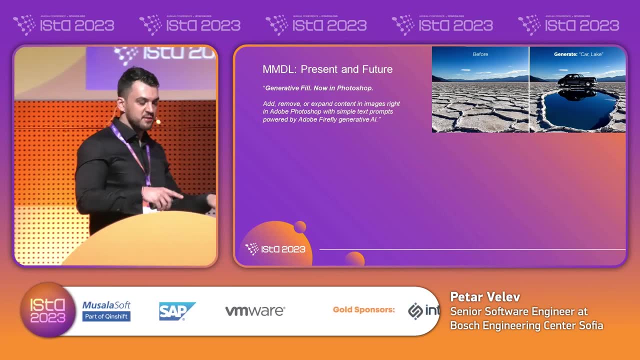 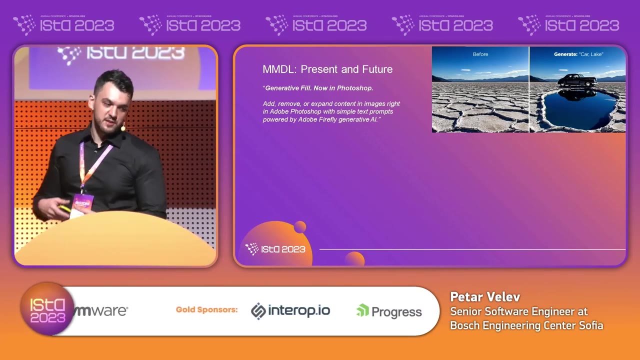 is generative, fill in Photoshop. This is a quote from their site. The idea behind it is that, for example, you can select a part of the image and then prompt the algorithm to generate a certain image inside it, and you need to try to preserve the uniqueness of the image. 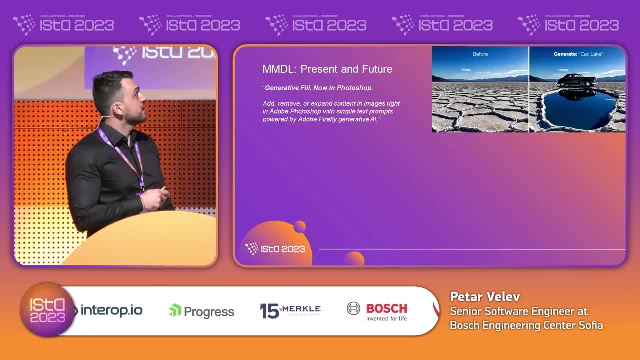 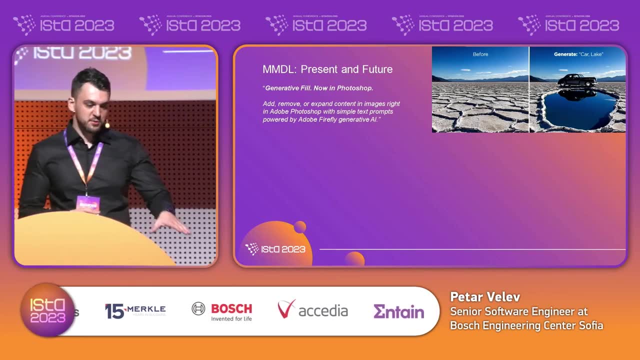 and the style of the image. And in this example that we see right here, for example, we ask the AI to generate the car and the lake, And what is interesting is that even in the lake there is the reflection of the car, so it does quite well. 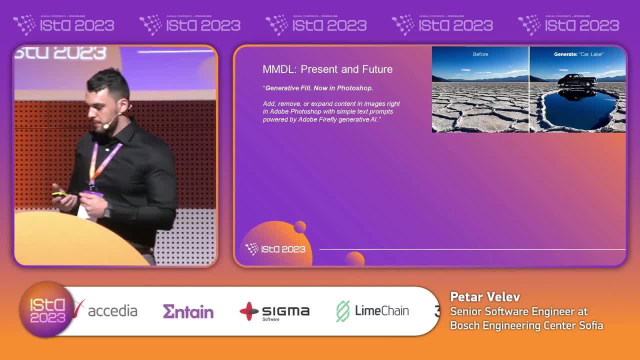 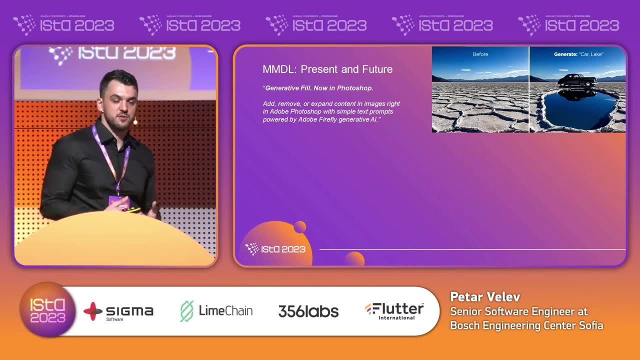 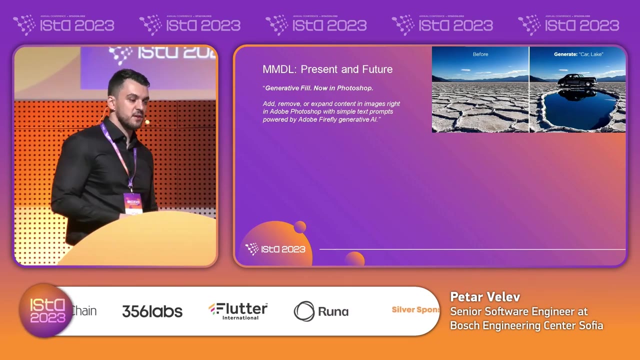 Another possible thing is, for example, view bird or visual bird, which is something that we pass an image and then we can prompt questions to this algorithm, For example, what's on that image or what will happen if we change something in that image? 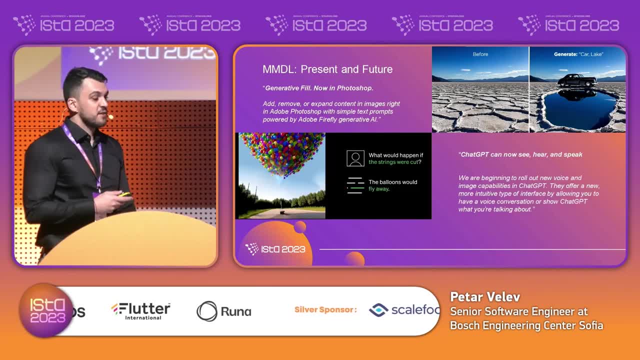 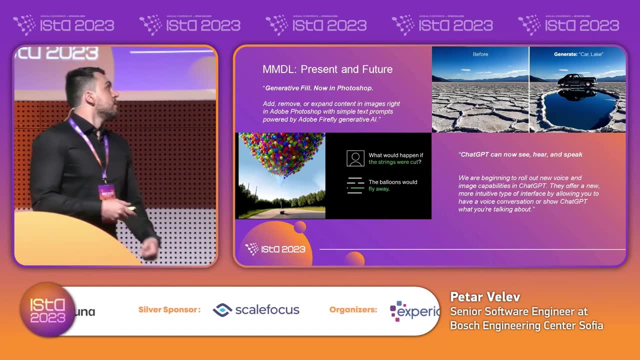 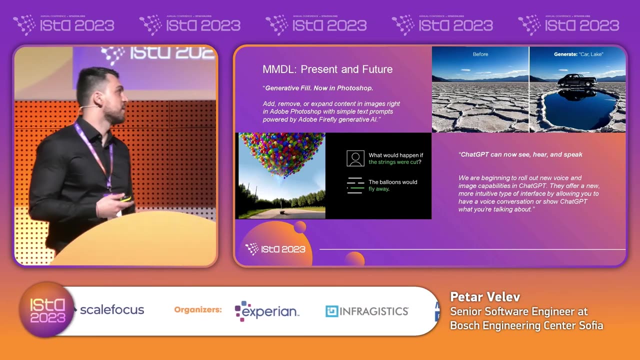 And, interestingly enough, this is something that will come to ChatGPT very soon, So this is also a quote from their site. They're beginning to roll out a new voice and image capabilities And, yeah, ChatGPT is becoming multi-model. 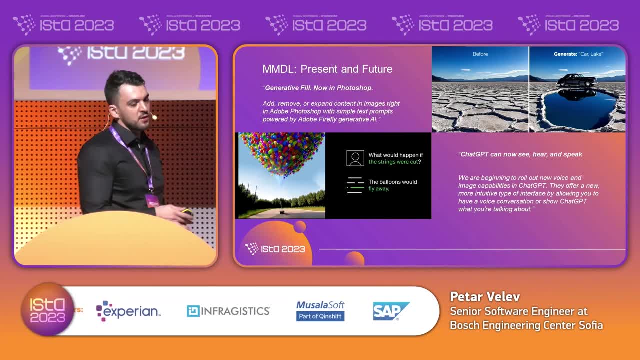 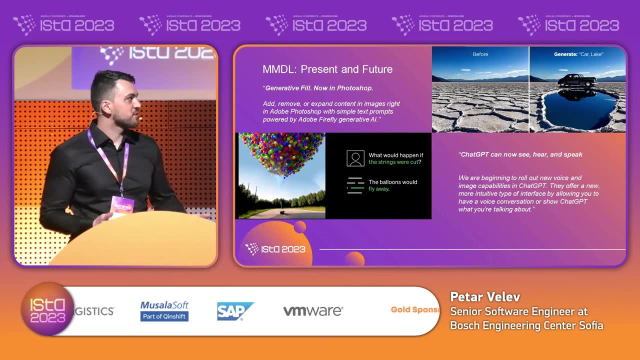 Apparently, we'll be able to, for example, take a picture of our car and our engine and then ask the algorithm to tell us how we can change the oil, for example. We need to generate a step-by-step guide on how to do it. 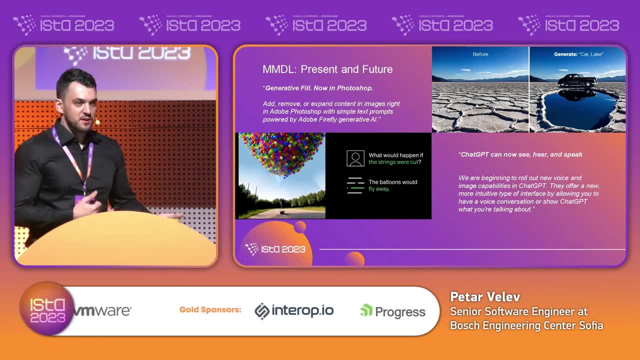 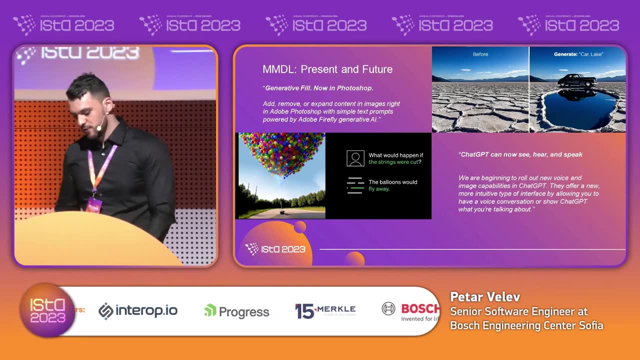 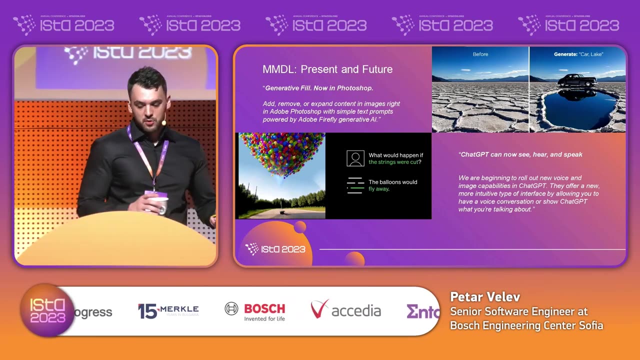 Or, for example, we can take a picture of ourselves and ask if this outfit sits okay on us, or something like that, And I'm wondering what is next. for example, I have this software. for example, DAUI. I don't know how many of you have heard about DAUI. 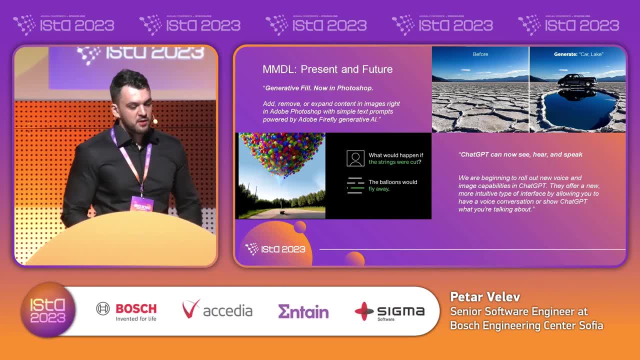 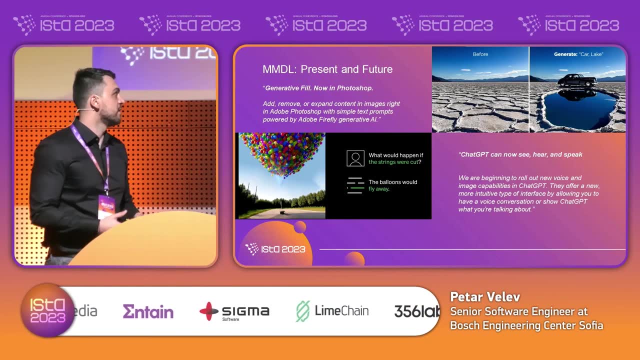 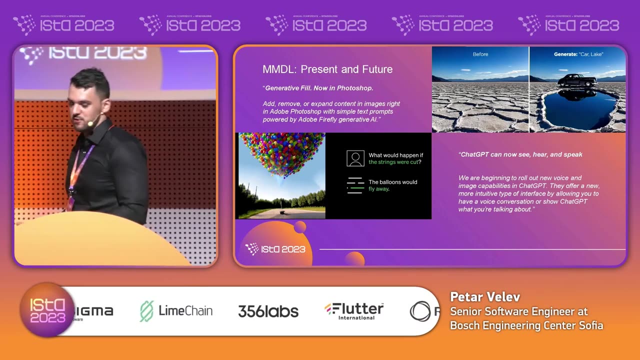 but it's a generative network which can generate images. So probably in the future they'll add this also to ChatGPT And there will be more and more modalities to this language model. that's ChatGPT right now, And where is the fine line that we'll draw? 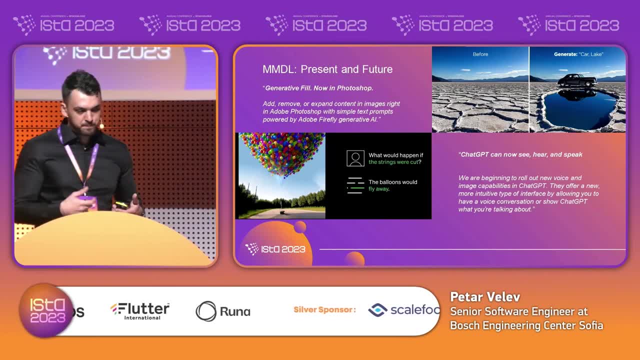 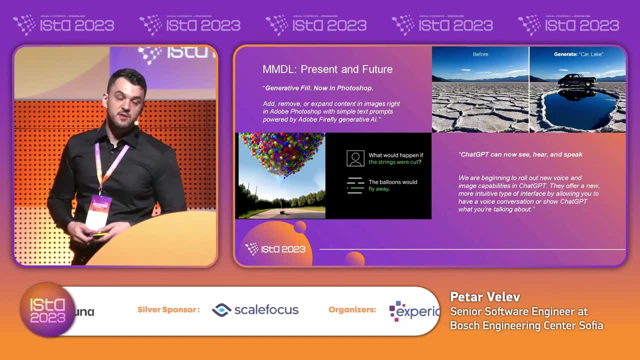 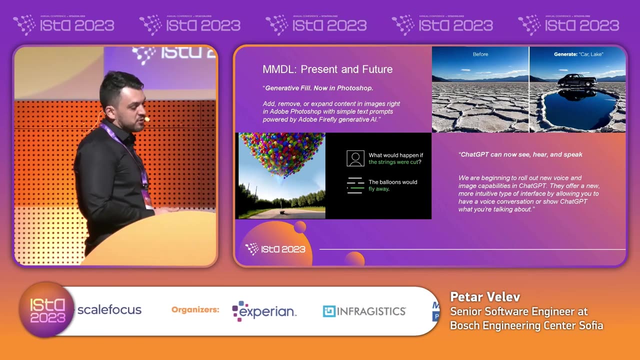 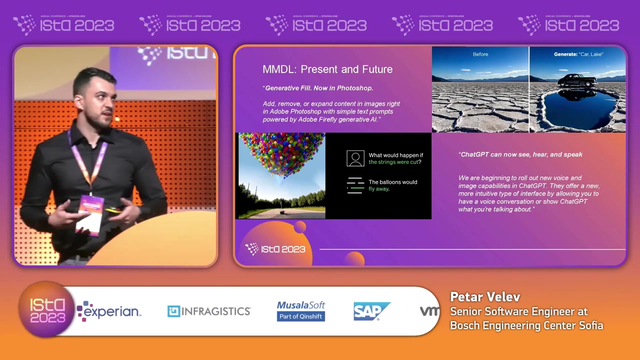 When this AI will become general and understand all of our information like humans understand it around us. Well, I personally don't know, But I think that multi-modality and multi-modal deep learning will be increasingly more popular And most of the newer developments in AI. 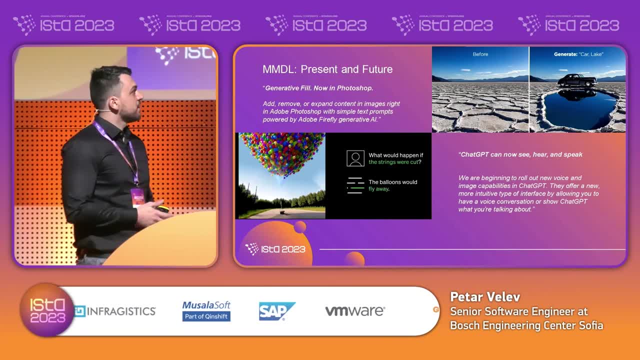 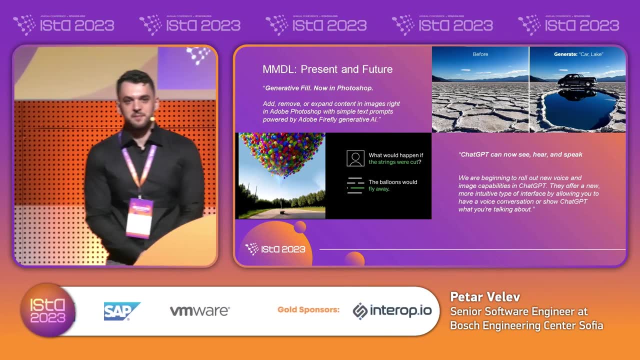 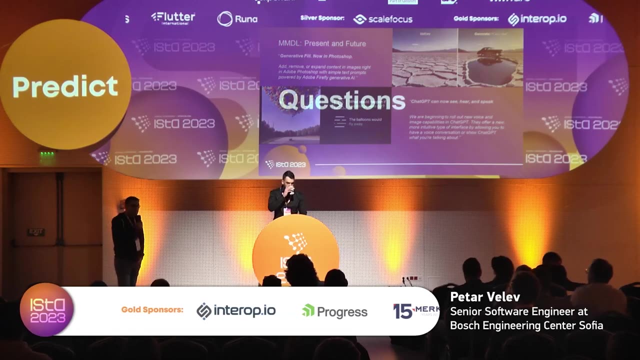 will be multi-modal, So hopefully today I was able to give you some introduction on this topic, or at least something of value. Thank you for your attention. Thank you, Peter. Do we have questions? I think we have like a couple more minutes. 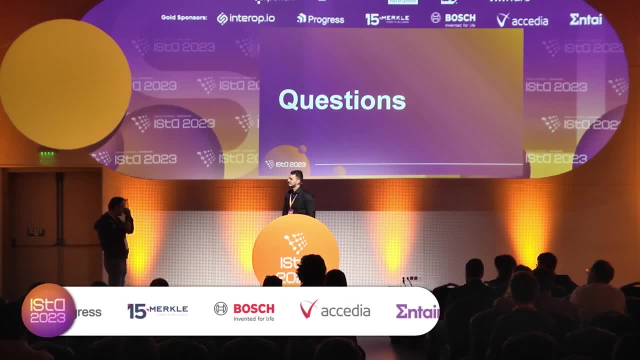 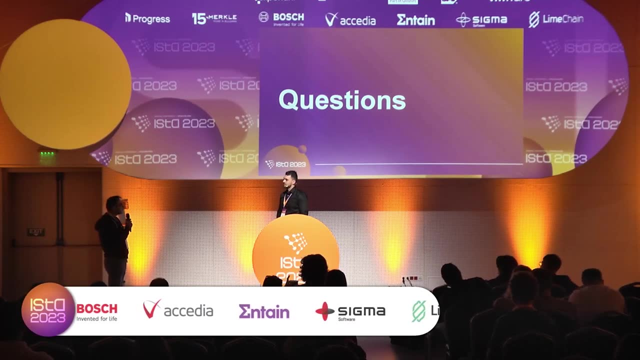 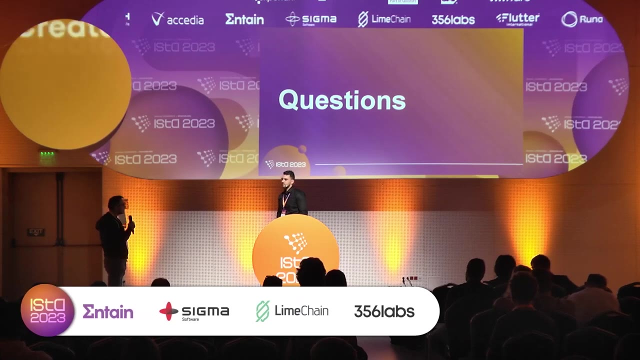 Okay, I have a question. actually, You mentioned the main challenges, So what are the when you start to think? in addressing these challenges, what are the standard approaches that are used there? No, it's quite difficult And it's a topic that is rapidly evolving. 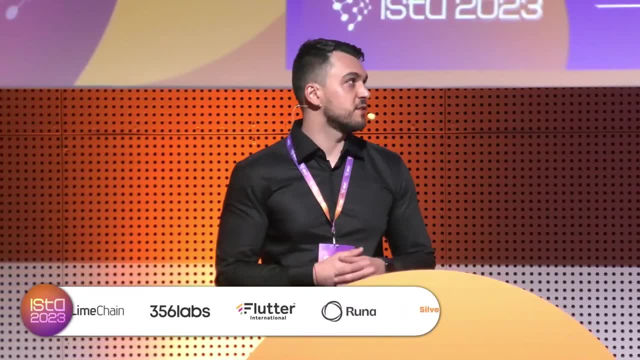 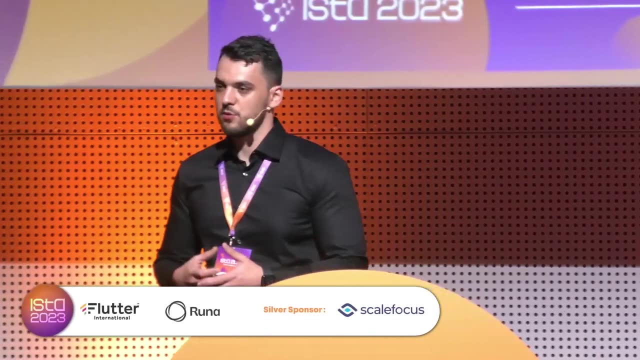 So there are certain ways to overcome these challenges. For example, as I said, data compatibility is one of the main things that we need before we design such algorithms, So we're trying to find a way that we can make these data, these data, compatible. 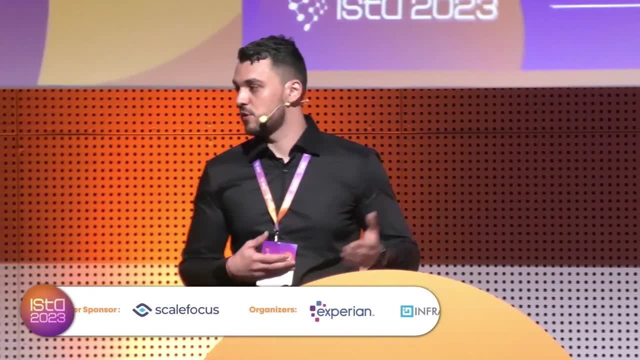 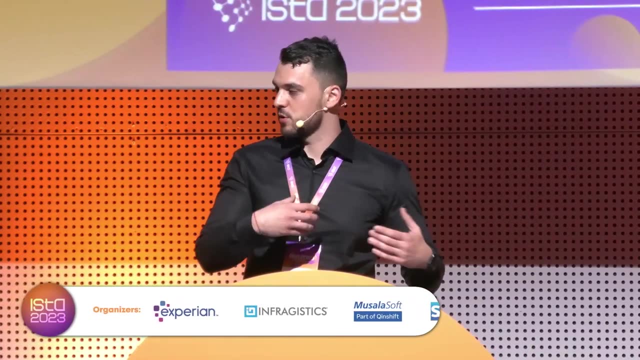 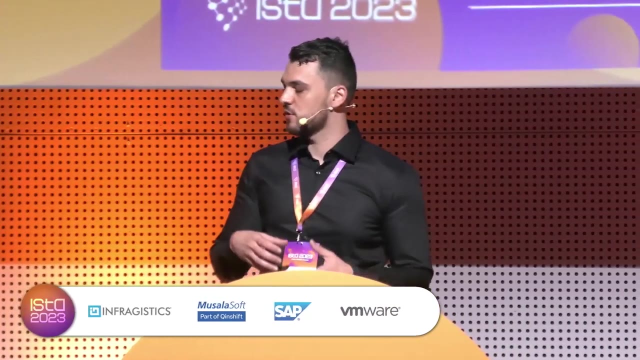 And this can be achieved, for example, like using some sort of an intermediate representation, where we normalize a layer of the network, for example, and combine it with something from the other model, or hierarchical fusion is something that combines, for example, features on very early stage. 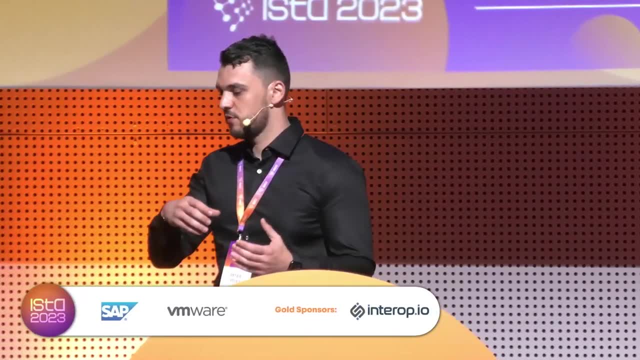 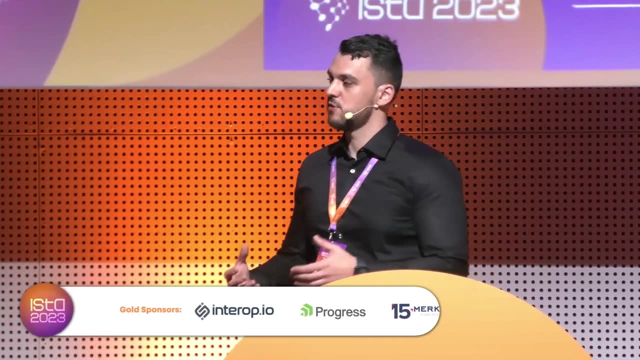 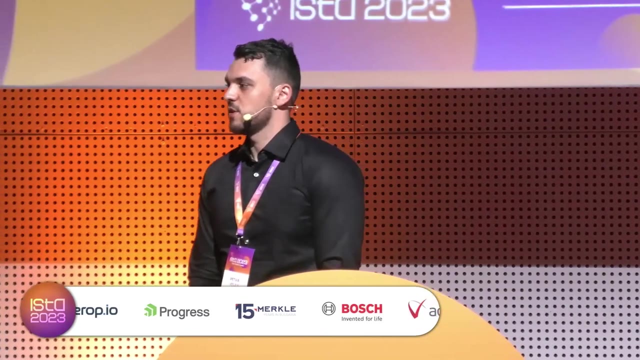 like the pixels from the image, with something that is very late, from other network, like the last layer of another network, and it normalizes this information and pass it later to another model. So there are different ways that can be used for achieving this. 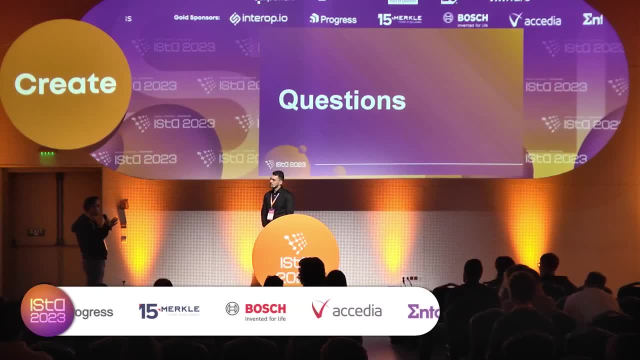 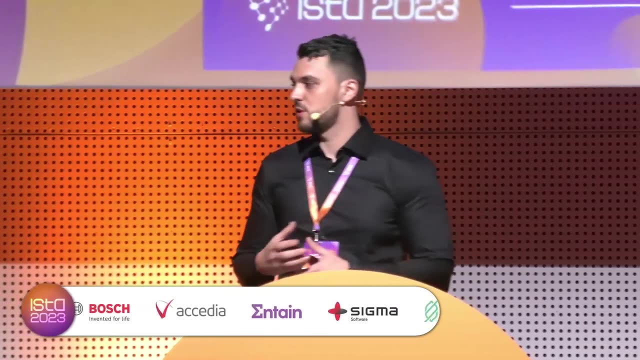 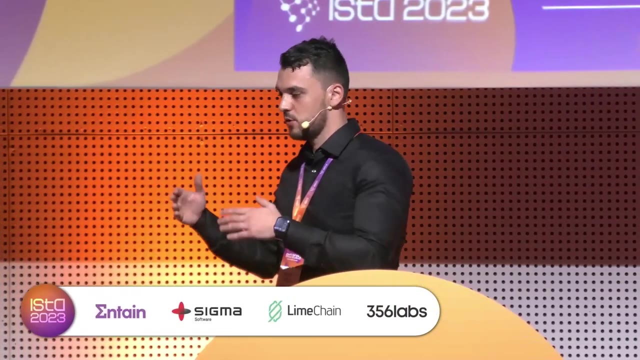 If I get it right, what you're trying to say is that you unify the characteristics of the data? Yeah, you're trying to make the data similar, because it's very difficult for the network to learn on different data, For example, if your values are normalized between zero and one. 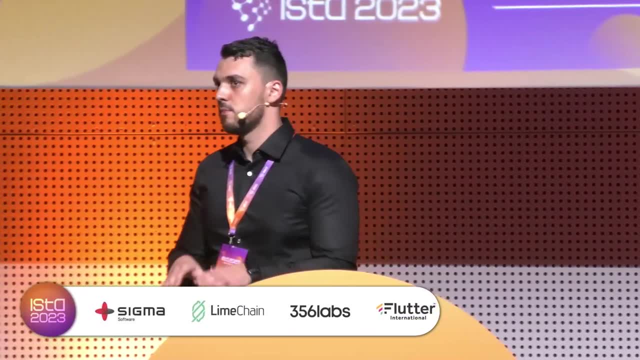 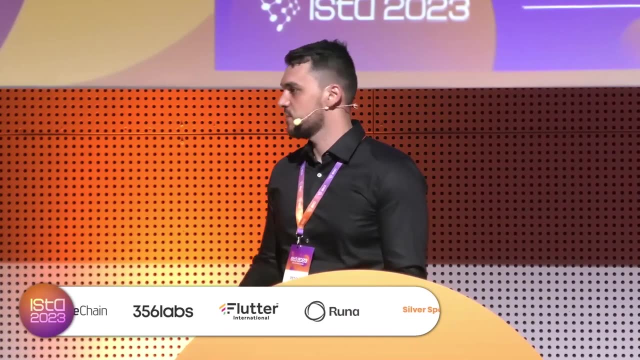 and all of these values are passed to the model, it will work. OK, maybe, But if the data is different- for example, one values are between zero and maxing, for example, and the other is some sort of normalized data between zero- 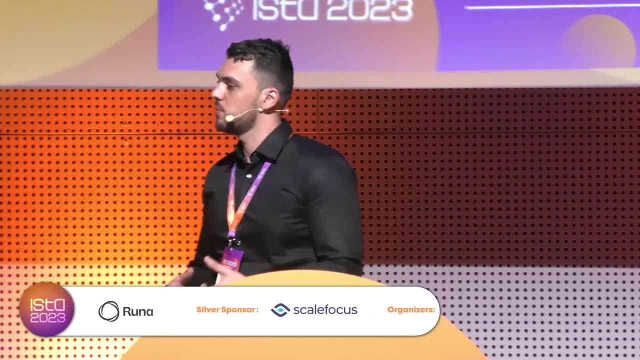 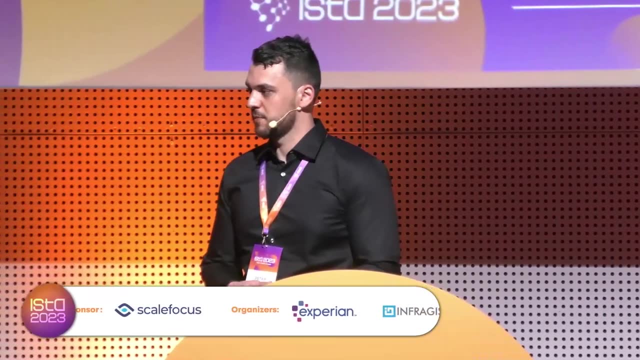 and one. it will be quite difficult for the network to adjust the weights, It will be difficult for the back propagation algorithm or the thing you're using to optimize the training, And I guess that the next step is probably data synchronization Or something else. 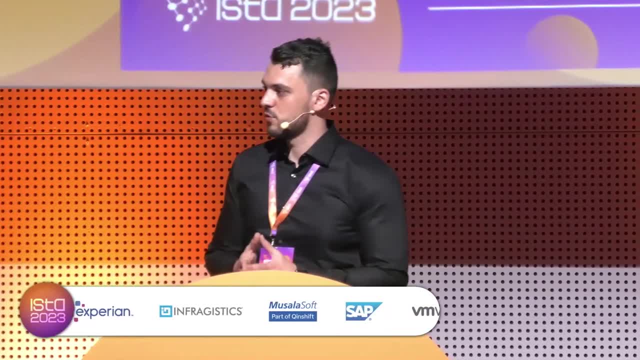 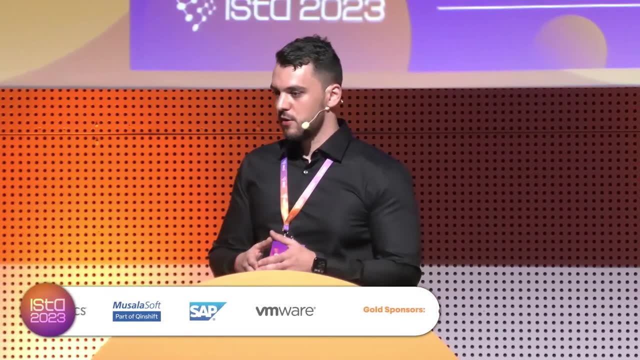 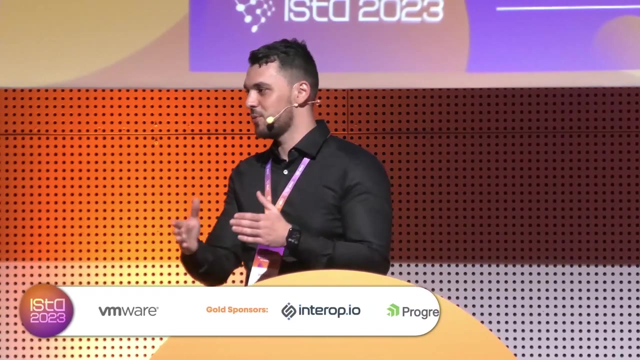 Actually, data synchronization is something that you need in your data set, for example. You need synchronized data in order to be able to teach the network certain stuff. For example, even for us humans, it's very difficult to like when you watch a video and the audio and video. 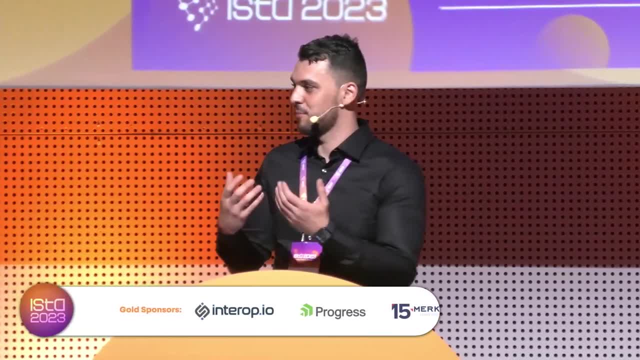 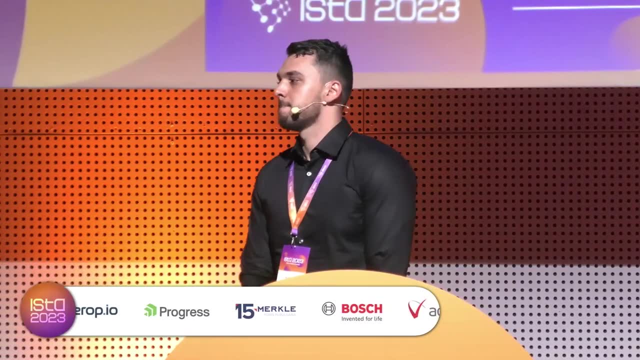 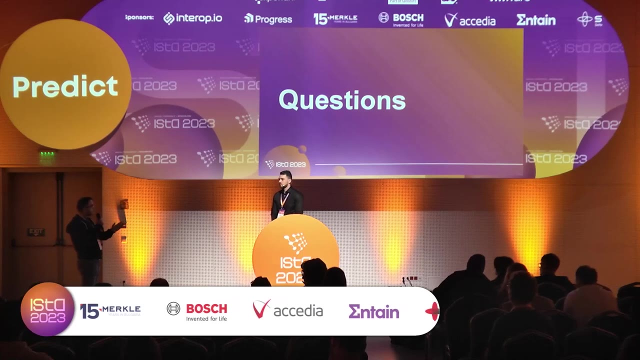 are kind of not synchronized. it's very difficult and it actually bugs us, So this is amplified when it comes to training neural networks. OK, just to confirm. these are the first steps in unifying the characteristics of the data, synchronizing them. 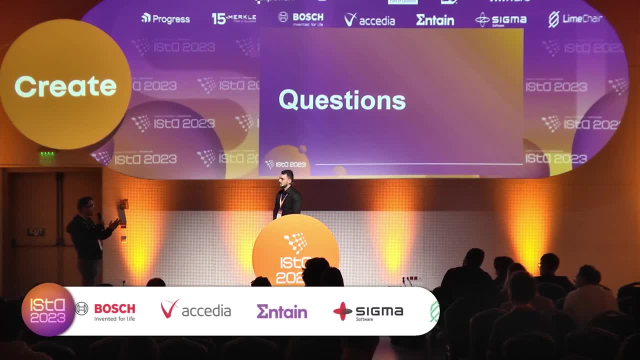 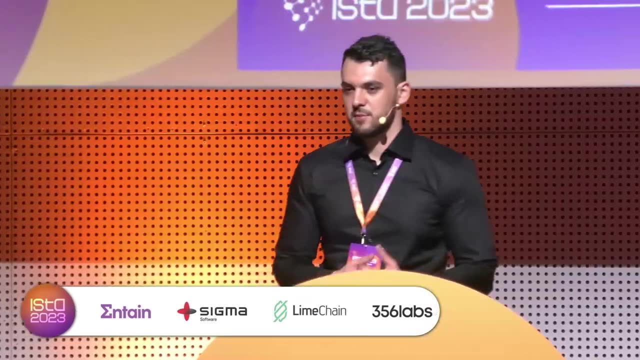 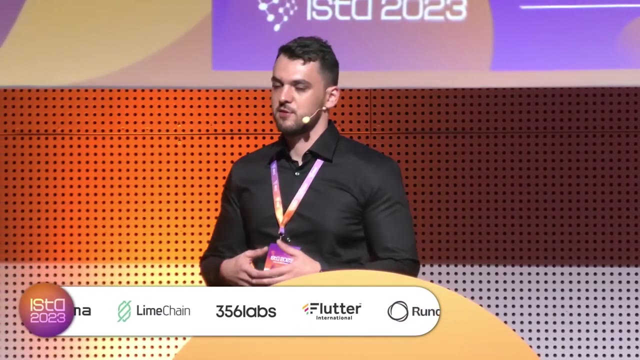 and the next step probably is building this. how do you call this approach for multi-modality? the different approaches that you mentioned early merge? Yeah, these are the basic approaches for fusing the data. There are a lot more approaches that can be used. 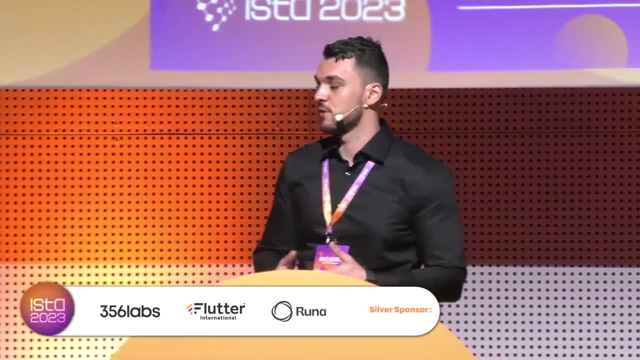 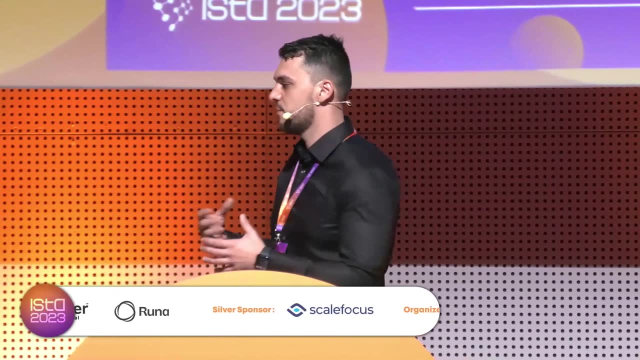 but it's quite difficult to go through all of them in such a short time and, to be honest, I don't know the insights of all of them. It's a field that rapidly evolves And I wouldn't say that this is the first step. 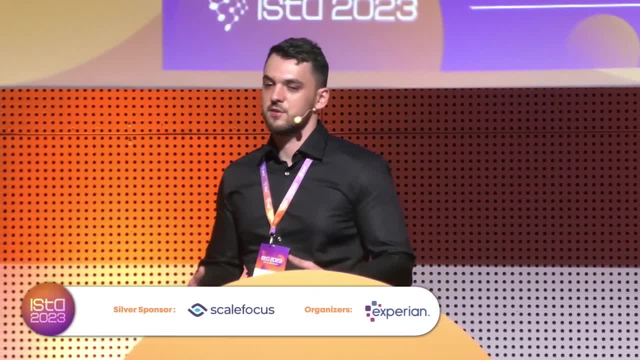 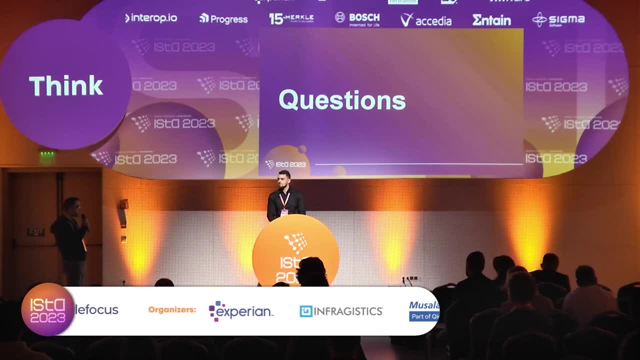 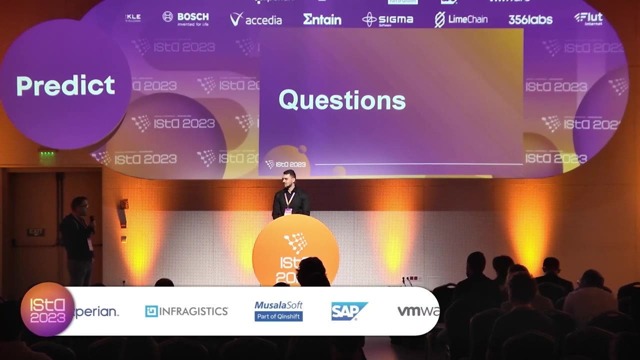 but this is one of the challenges in training such a multi-modal systems. Data synchronization is one of the challenges. Yeah, thank you. This definitely. your talk is like an introduction, so everyone who is interested can deep dive and get more details. 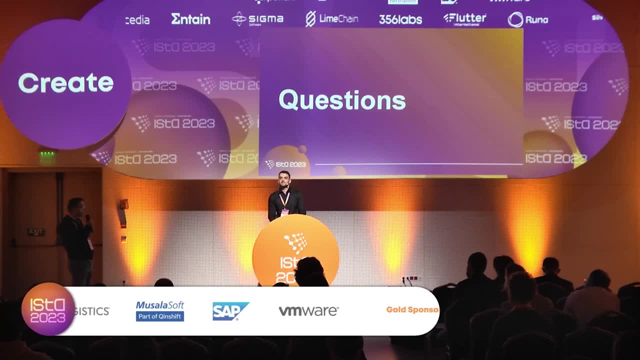 Do we have other questions? No, well, thank you Peter. Thank you.